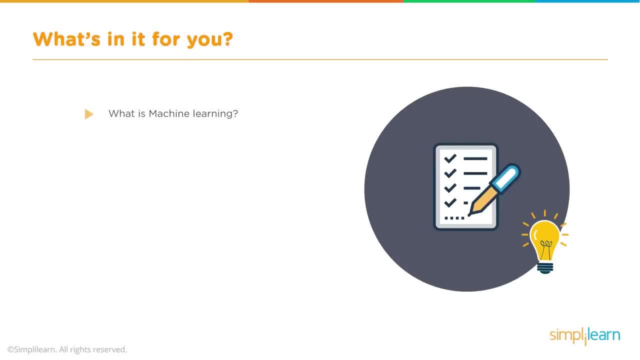 what you would want to use some other tools for. What's in it for you? Today we're going to cover about six different sections. We're going to start with what is machine learning, so we can see where the vector machine fits in. why the Support Vector Machine? what is a Support Vector Machine and 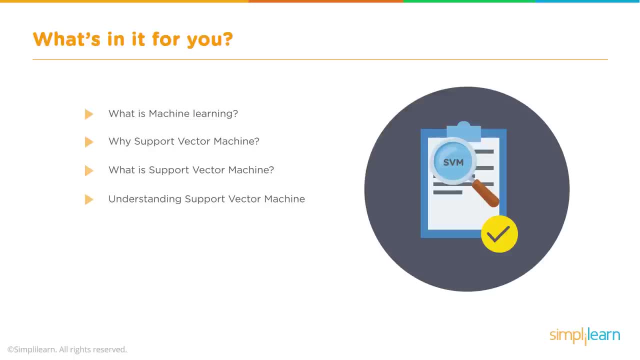 understanding the Support Vector Machine. Once we go through an understanding of how it works and what it looks like, we're going to look at the advantages of Support Vector Machine and finally dive into a use case in Python where we'll write some script on it. Let's start with what is machine. 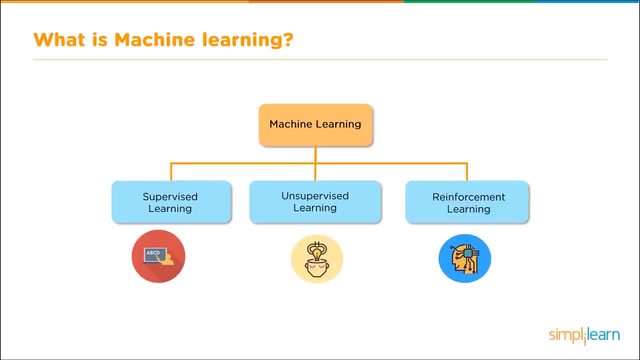 learning and, even more specific, where does the Support Vector, Machine algorithm, fit in? The biggest split in machine learning is between the three categories: supervised learning, where we have data and we can train it. unsupervised learning, where we're just guessing at what we. 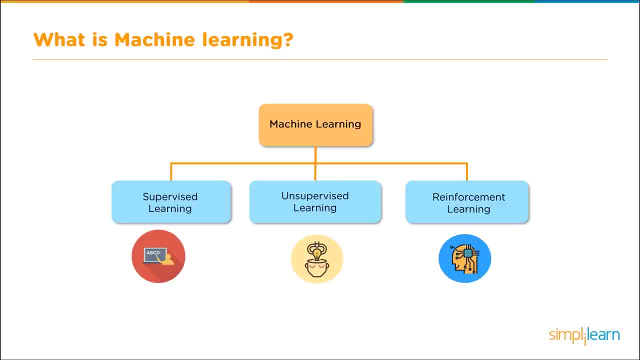 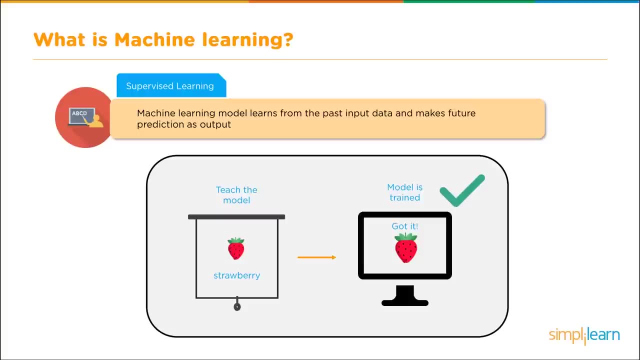 can make sense of the data and reinforcement learning where we reinforce a good or bad behavior. Since the SVM is specific to supervised learning, machine learning model learns from the past input data and makes future predictions as output. So we teach the model, we teach it. what a 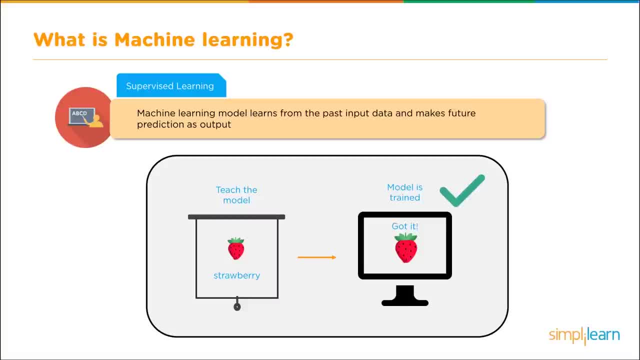 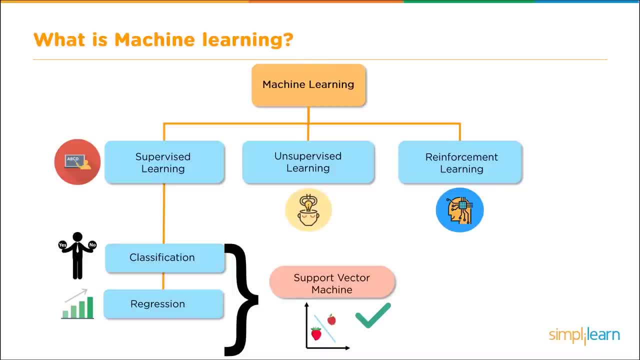 strawberry is, and once the model is trained, it can identify a strawberry. That's what's meant by supervised learning In the larger picture of the machine learning model and under supervised learning, you can see that the support vector fits in under classification, deciding what. 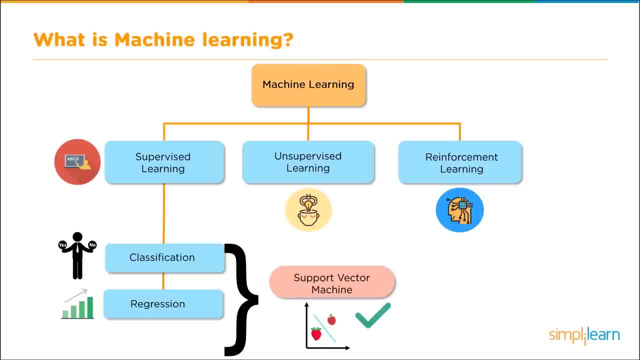 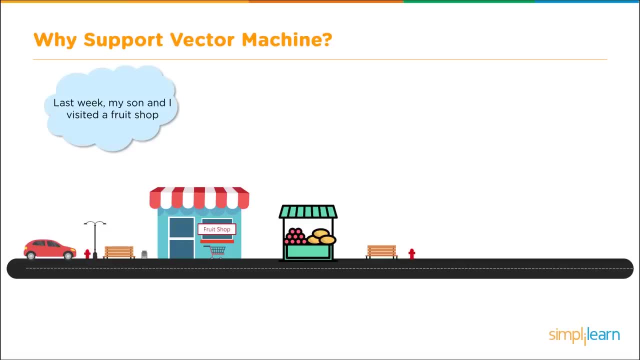 yes and no is, And there is also a regression version, but it is primarily used for classification. Let's take a detour and see if we can connect this to the human experience and find out why. support vector machine. So in this example, last week my son and I visited a fruit shop. Dad is 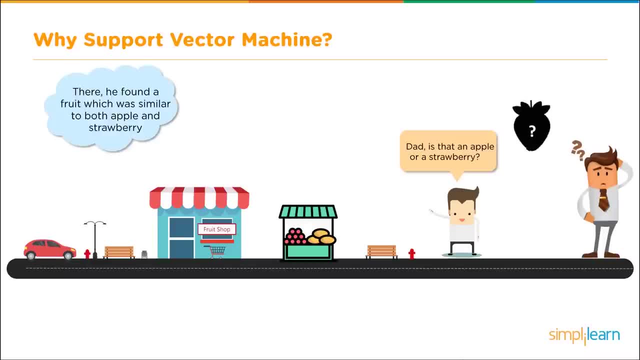 that an apple or a strawberry? So the question comes up: what fruit did I just pick up from the fruit stand? After a couple of seconds, you can figure out that it was a strawberry. So let's take this model a step further and let's- why not, build a model which can predict an unknown data. 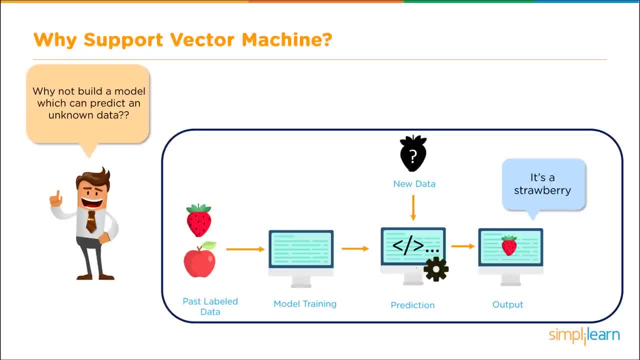 And in this we're going to be looking at some sweet strawberries or crispy apples. We want it to be able to label those two and decide what the fruit is, And we do that by having data already put in. So we already have a bunch of strawberries we know are strawberries and they're. 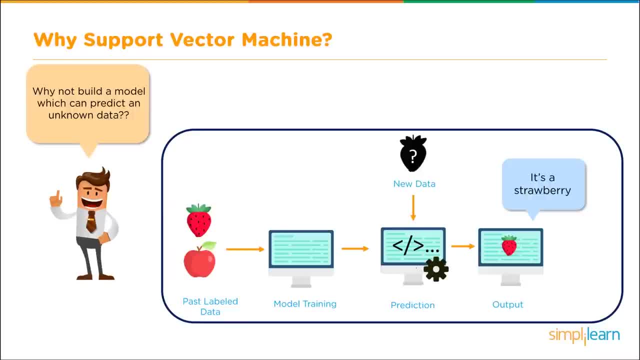 already labeled as such. We already have a bunch of apples we know are apples and are labeled as such. Then, once we train our model, that model then can be given the new data. and the new data is this image. In this case, you can see a question mark on it and it comes through and goes: it's a strawberry. 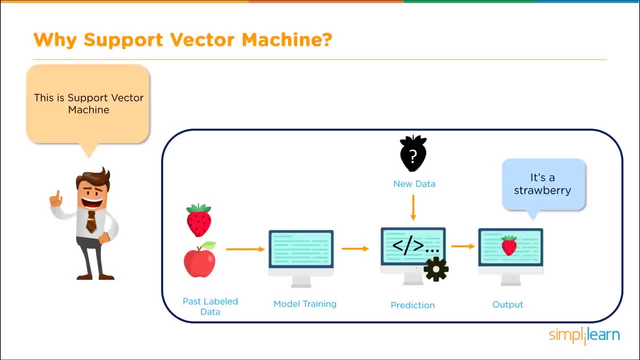 In this case we're using the support vector machine model. SVM is a supervised learning method that looks at data and it's going to be able to predict what's going to happen. So we want that data and sorts it into one of two categories, And in this case we're sorting the strawberry. 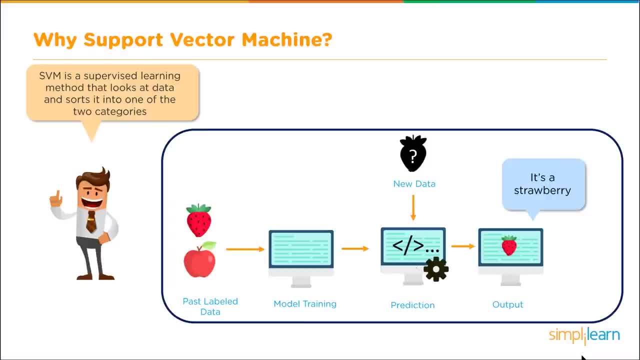 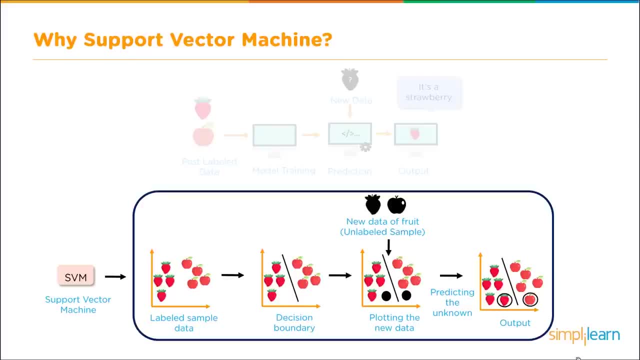 into the strawberry side. At this point you should be asking the question: how does the prediction work? Before we dig into an example with numbers, let's apply this to our fruit scenario. We have our support vector machine, We've taken it and we've taken labeled sample. 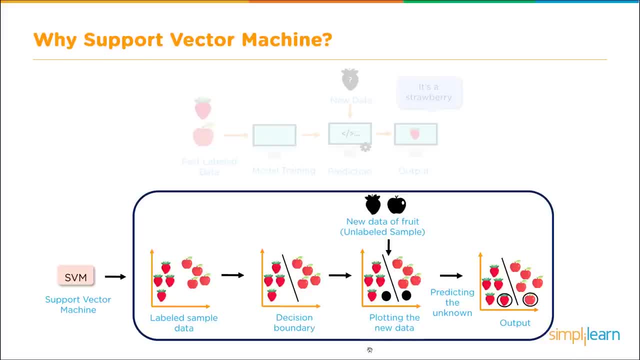 of data- strawberries and apples- and we draw on a line down the middle between the two groups. This split now allows us to take new data- in this case an apple and a strawberry- and place them in the appropriate group based on which side of the line they fall in, And 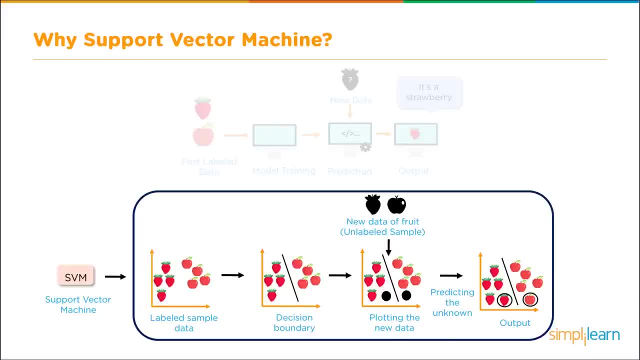 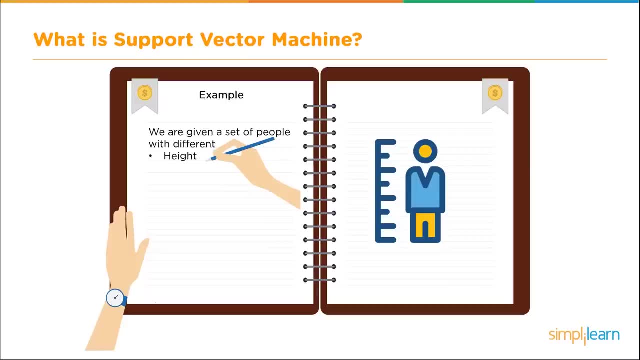 that way, we can predict the unknown. As colorful and tasty as the fruit example is, let's take a look at another example with some numbers involved And we can take a closer look at how the math works. In this example, we're going to be classifying men and women, And 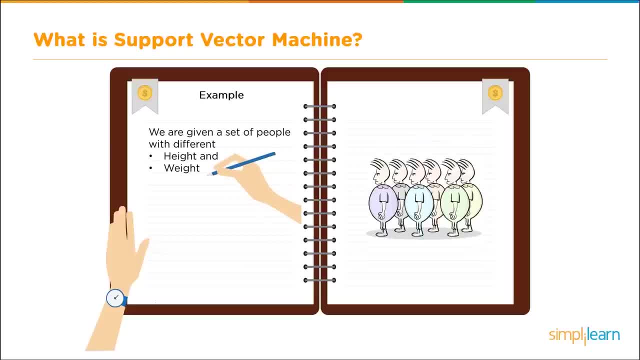 we're going to start with a set of people with a different height and a different weight And to make this work we'll have to have a sample data And we're going to have to have a sample data set of female, where you have their height and weight: 174,, 65,, 174,. 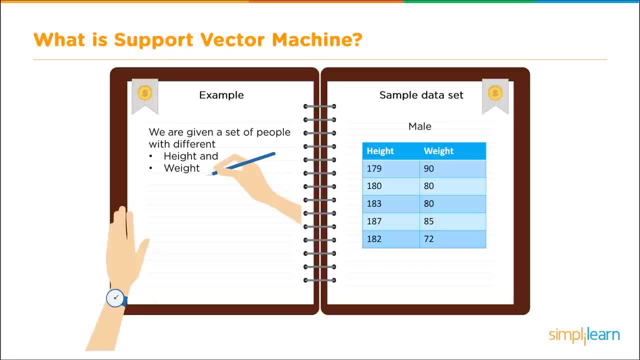 88, and so on, And we'll need a sample data set of the male. They have a height: 179,, 90,, 180 to 80, and so on. Let's go ahead and put this on a graph, so we have a nice visual. 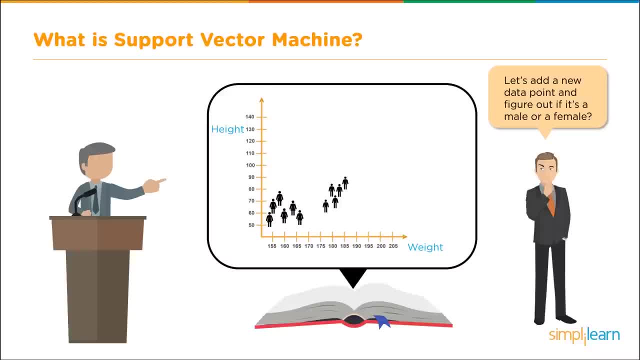 So you can see, here we have two groups based on the height versus the weight, And on the left side we're going to have the women, On the right side we're going to have the men. Now, if we're going to create a classifier, let's add a new data point and figure out. 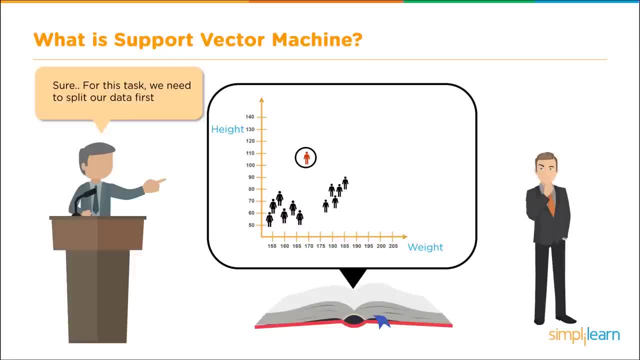 if it's male or female. But we need to split our data first. We can split our data by choosing any of these lines. In this case, we've drawn two lines through the data in the middle. that separates the men from the women. But to predict the gender of a new data point, we should split the data. 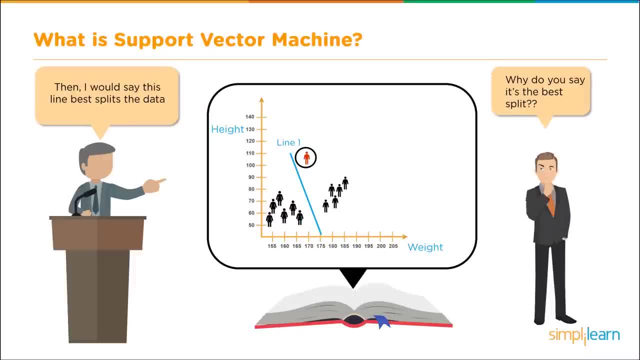 in the best possible way. And we say the best possible way because this line has a maximum space that separates the two classes. Here you can see there's a clear split between the two different classes, And in this one there's not so much a clear split. 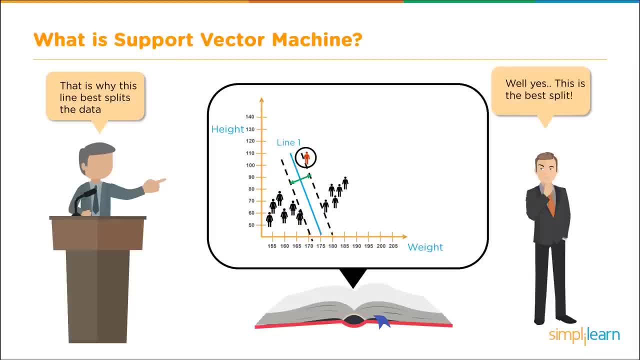 This doesn't have the maximum space that separates the two. That is why this line best splits the data. We don't want to just do this by eyeballing it, And before we go further, we need to add some technical terms to this. We can also say that the distance between 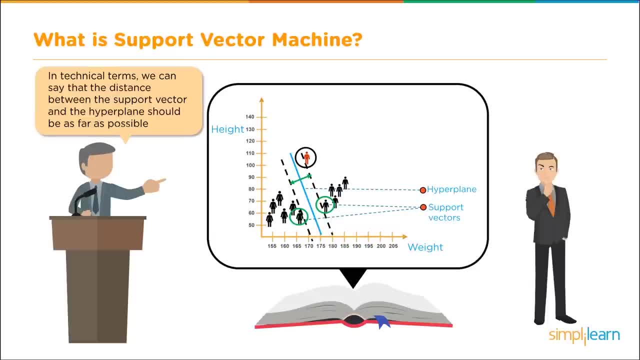 the points in the line should be as far as possible. In technical terms we can say the distance between the support vector and the hyperplane should be as far as possible, And this is where the support vectors are the extreme points in the dataset. And if you 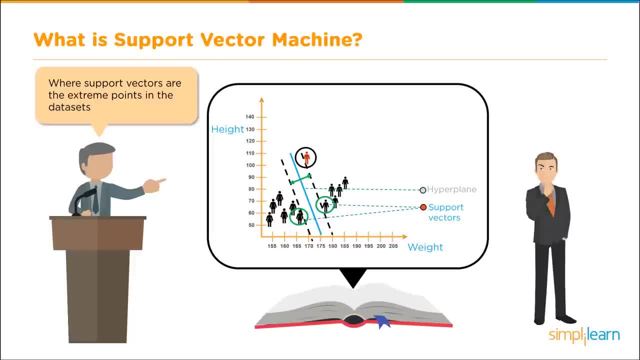 look at this dataset, They have circled two points which seem to be right on the outskirts of the women and one on the outskirts of the men, And hyperplane has a maximum distance to the support vectors of any class. Now you'll see the line down the middle and we call this the hyperplane, because when you're dealing with multiple dimensions, 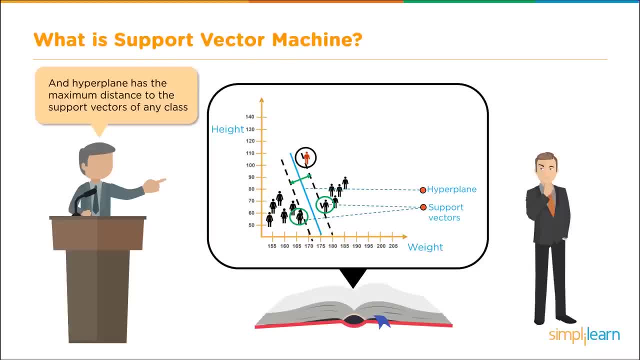 it's really not just a line but a plane of intersections, And you can see here where the support vectors have been drawn in dashed lines. The math behind this is very simple: We take d plus the shortest distance to the closest positive point, which would be on the men's side. 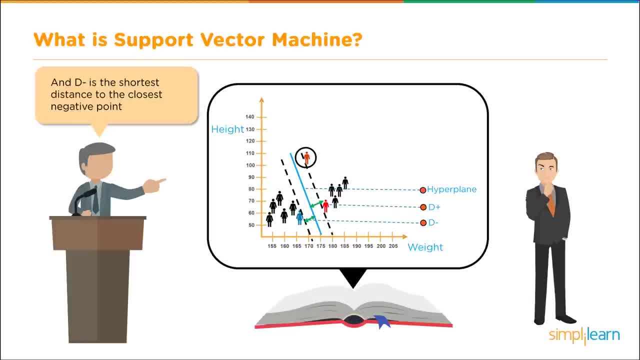 and d minus is the shortest distance to the closest negative point, which is on the women's side. The sum of d plus and d minus is called the distance margin, or the distance between the two support vectors that are shown in the dashed lines. 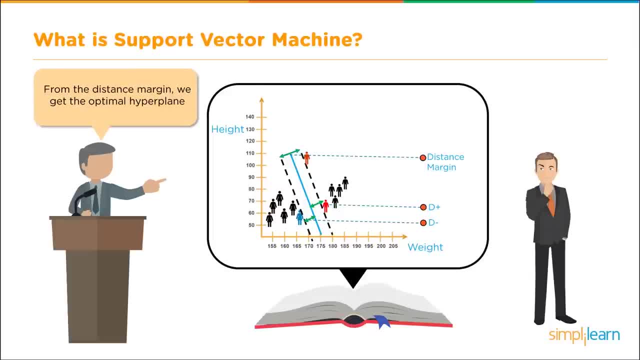 And then, by finding the largest distance margin, we can get the optimal hyperplane. Once we've created an optimal hyperplane, we can easily see which side the new data fits in And based on the hyperplane, we can say the new data point belongs to the male gender. 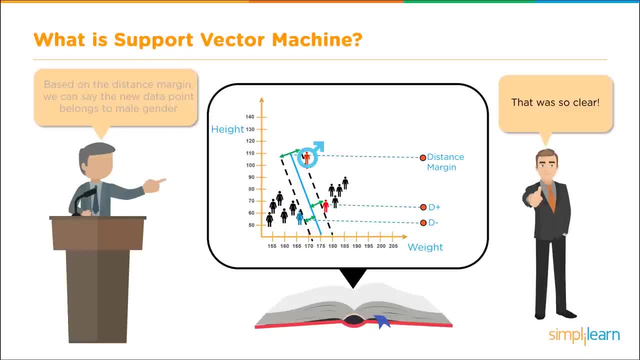 Hopefully that's clear how that works on a visual level. As a data scientist, you should also be asking what happens if the hyperplane is not optimal. If we select a hyperplane having low margin, then there is a high chance of misclassification. 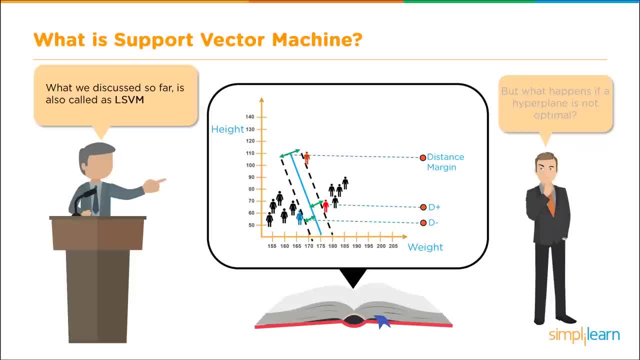 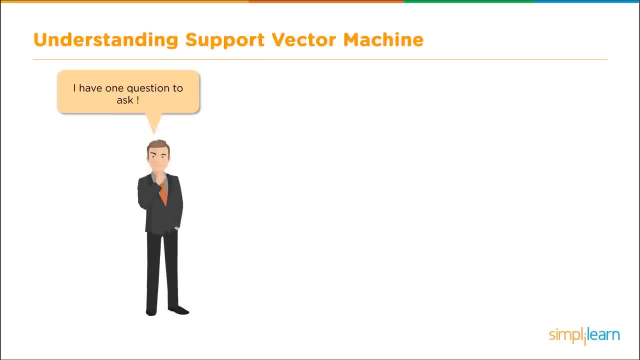 This particular SVM model, the one we discussed so far, is also called or referred to as the LSVM. So far, so clear. but a question should be coming up. We have our sample data set, But instead of looking like this, what if it looked like this? 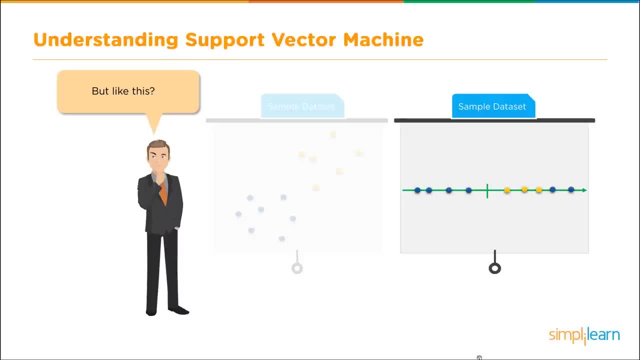 where we have two sets of data but one of them occurs in the middle of another set. You can see here where we have the blue and the yellow and then blue again on the other side of our data line. In this data set we can't use a hyperplane. 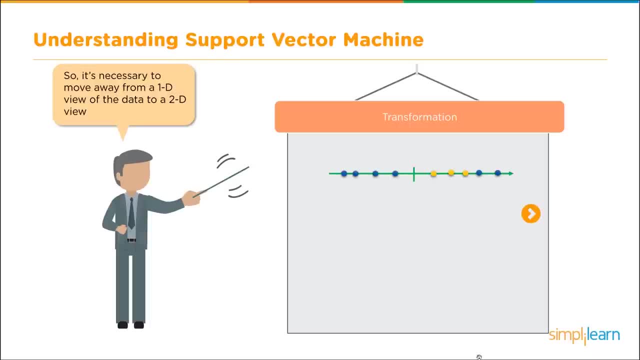 So when you see data like this, it's necessary to move away from a 1D view of the data to a two-dimensional view of the data, And for the transformation we use what's called a kernel function. The kernel function will take the 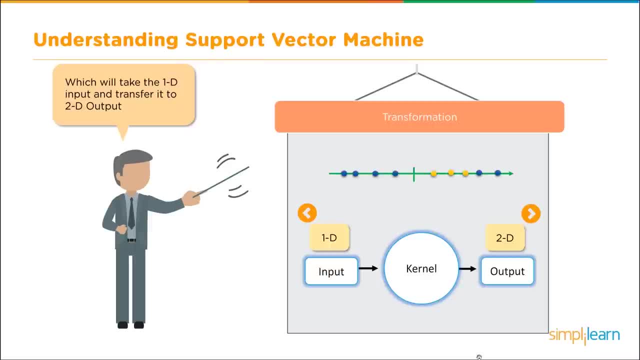 1D input and transfer it to a two-dimensional output. As you can see in this picture here, the 1D, when transferred to a two-dimensional, makes it very easy to draw a line between the two data sets. What if we make it even more complicated? 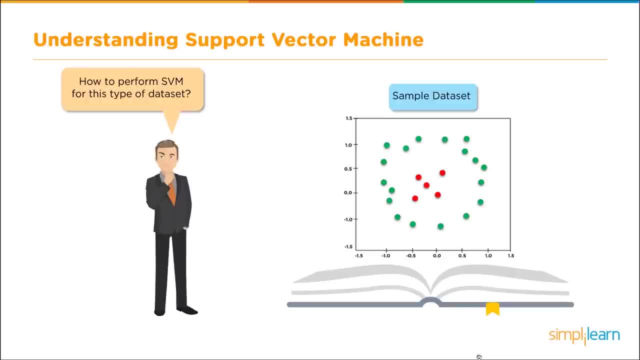 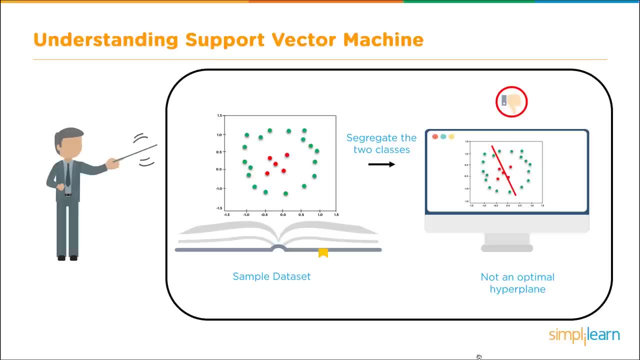 How do we perform an SVM for this type of data set? Here you can see, we have a two-dimensional data set where the data is in the middle surrounded by the green data on the outside. In this case, we're going to segregate the two classes. 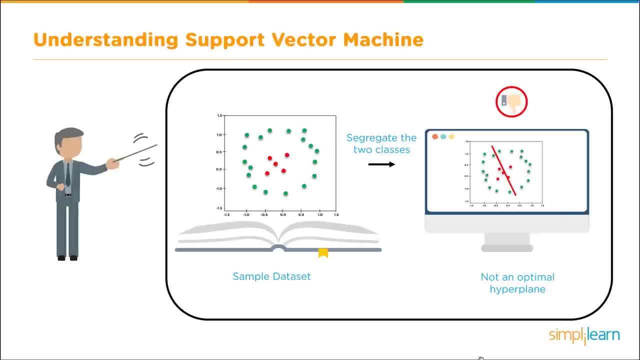 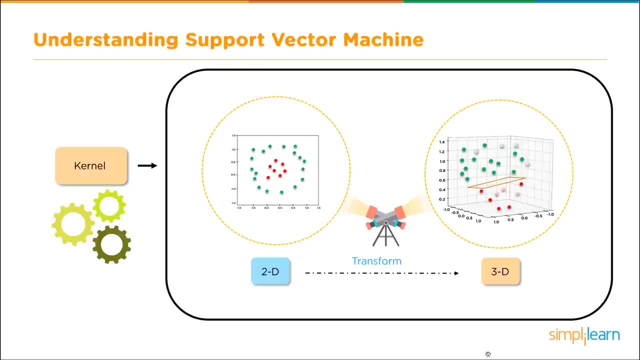 We have our sample data set And if you draw a line through it's obviously not an optimal hyperplane in there. So to do that we need to transfer the 2D to a 3D array And when you translate it into a three-dimensional array using the kernel. 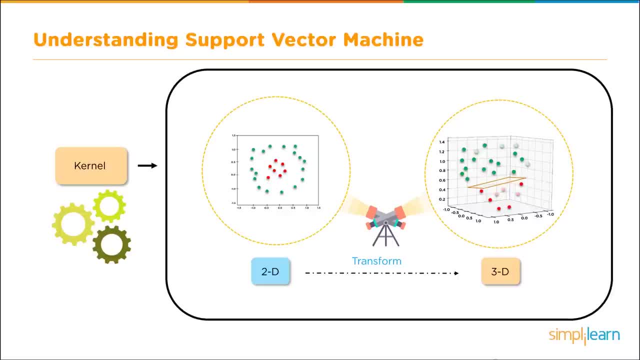 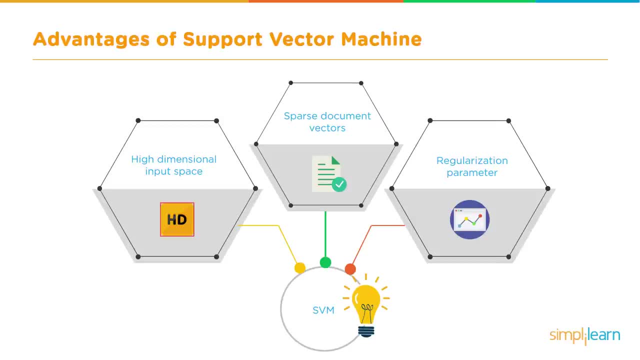 you can see where you can place a hyperplane right through it and easily split the data. Before we start looking at a programming example and dive into the script, let's look at the advantage of the support vector machine. We'll start with high-dimensional input space. 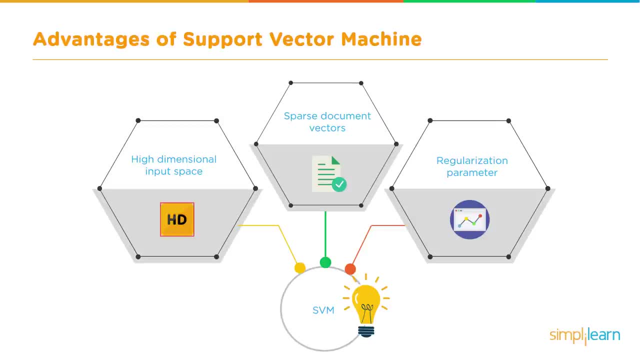 or sometimes referred to as the curse of dimensionality We looked at earlier one-dimension, two-dimension, three-dimension. When you get to a thousand dimensions, a lot of problems start occurring with most algorithms that have to be adjusted for. 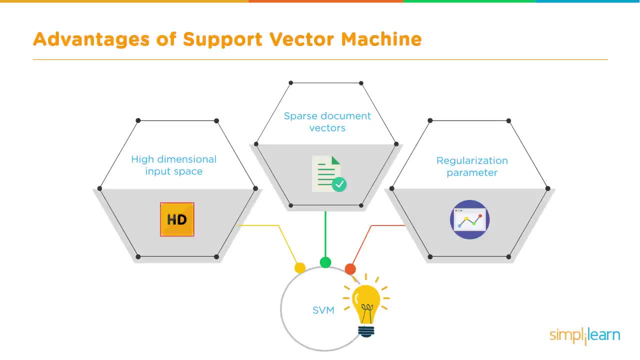 The SVM automatically does that in high-dimensional space. One of the high-dimensional space, one high-dimensional space that we work on, is sparse document vectors. This is where we tokenize the words and documents so we can run our machine learning algorithms over them. I've seen ones get as high as 2.4 million different tokens. 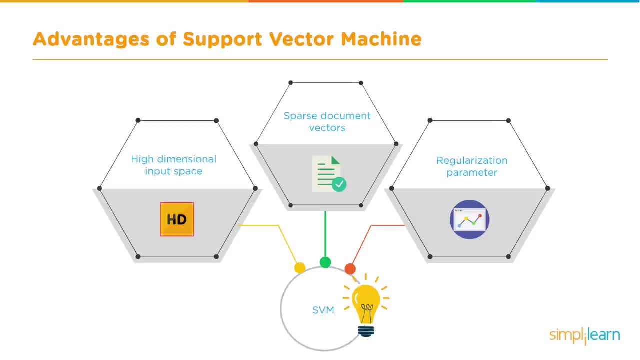 That's a lot of vectors to look at. And finally, we have regularization parameter. The regularization parameter, or lambda, is a parameter that helps figure out whether we're going to have a bias or overfitting of the data, Whether it's going to be overfitted to a very specific instance or it's going to be biased to a high or low value. 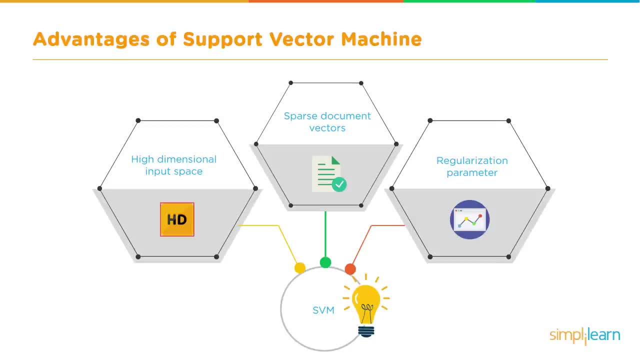 With the SVM, it naturally avoids the overfitting and bias problems that we see in many other algorithms. These three advantages of the support vector machine make it a very powerful tool to add to your repertoire of machine learning tools. Now we did promise you a use case study. 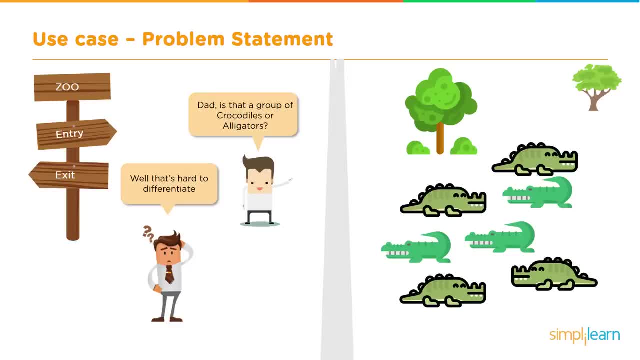 We're actually going to dive in To some Python programming And so we're going to go into a problem statement and start off with the zoo. So in the zoo example we have family members going to the zoo, We have the young child going, Dad, is that a group of crocodiles or alligators? 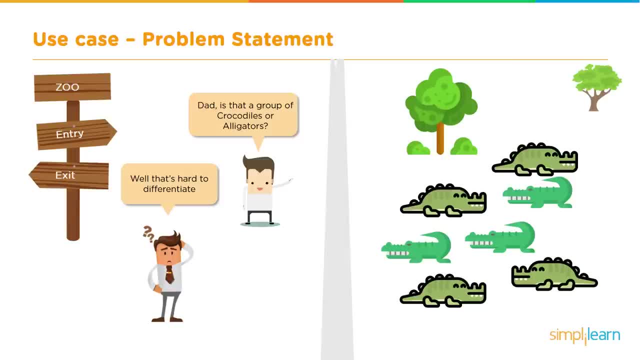 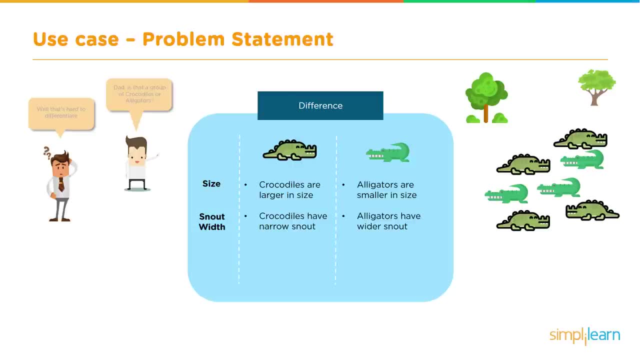 Well, that's hard to differentiate, And zoos are a great place to start looking at science and understanding how things work, especially as a young child. And so we can see the parents sitting here thinking: well, what is the difference between a crocodile and an alligator? 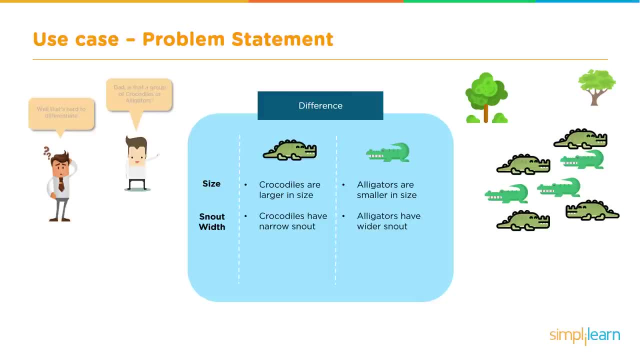 Well one, crocodiles are larger in size, Alligators are smaller in size. Snout width: the crocodiles have a narrow snout and alligators have a wider snout. And of course, in the modern day and age, the father sitting here is thinking: how can I turn this into a lesson for my son? 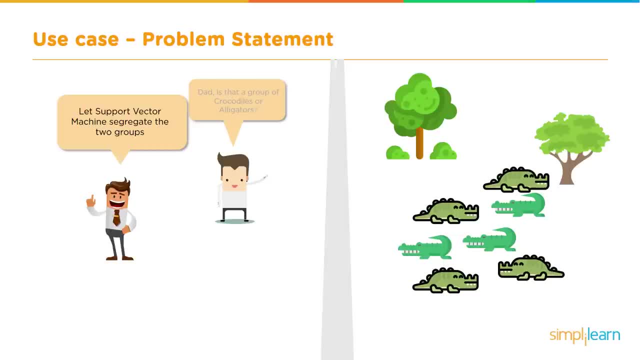 And he goes, let a support vector machine segregate the two groups. I don't know if my dad ever told me that, but that would be funny. Now, in this example, we're not going to use actual measurements and data. We're just using that for imagery. 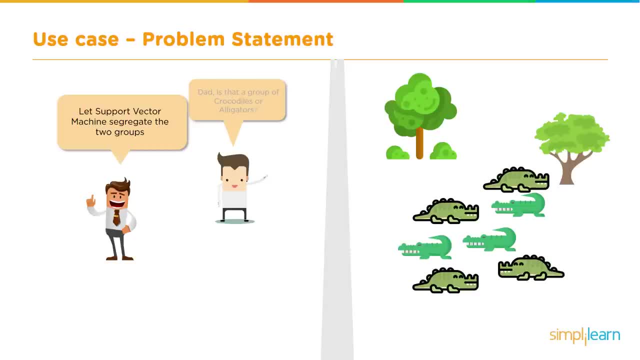 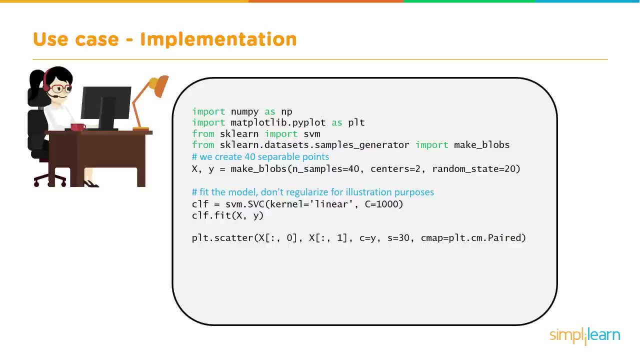 And that's very common in a lot of machine learning algorithms- and setting them up. But let's roll up our sleeves- and we'll talk about that more in just a moment- as we break into our Python script. So here we arrive, in our actual coding. 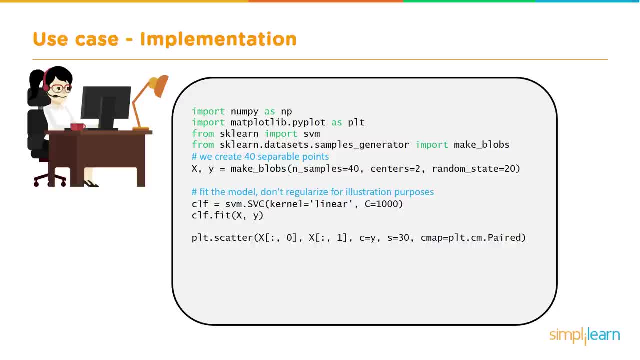 And I'm going to move this into a Python editor in just a moment. But let's talk a little bit about what we're going to cover First. we're going to cover in the code the setup, how to actually create our SVM. 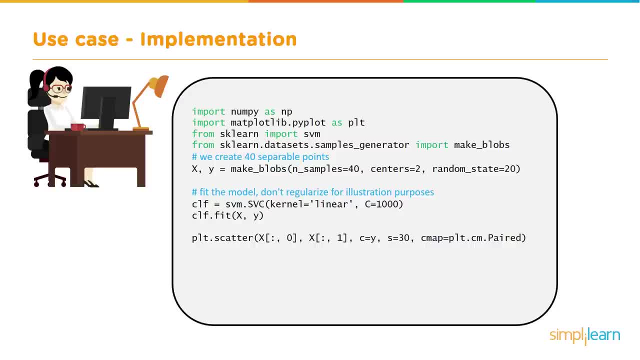 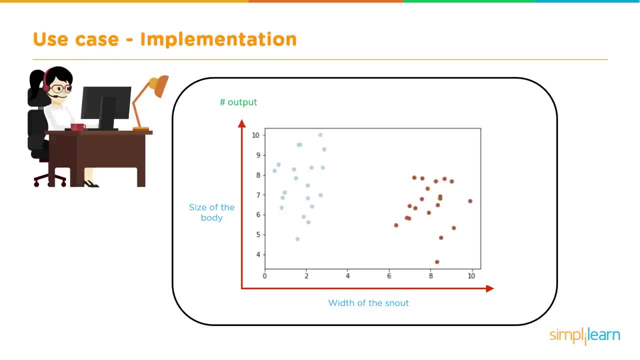 And you're going to find that there's only two lines of code that actually create it, And the rest of it is done so quick and fast that it's all here in the first page, And we'll show you what that looks like as far as our data, because we're going to create some data. 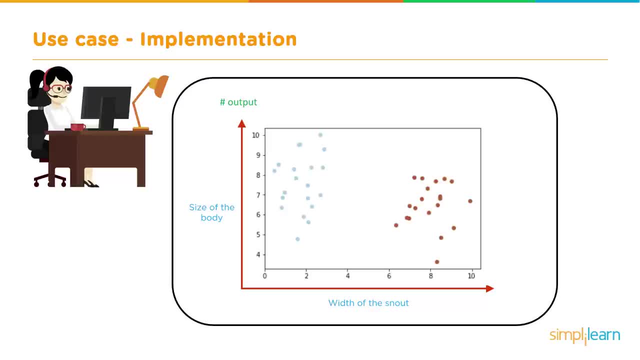 I talked about creating data just a minute ago, And so we'll get into the creating data here And you'll see this nice correction of our two blobs And we'll go through that in just a second. And then the second part is we're going to take this and we're going to bump it up a notch. 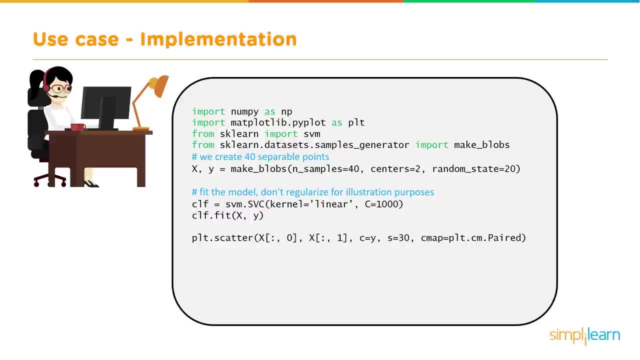 We're going to show you what it looks like behind the scenes, But let's start with actually creating our setup. I like to use the Anaconda Jupyter notebook because it's very easy to use, But you can use any of your favorite Python editors or setups and go in there. 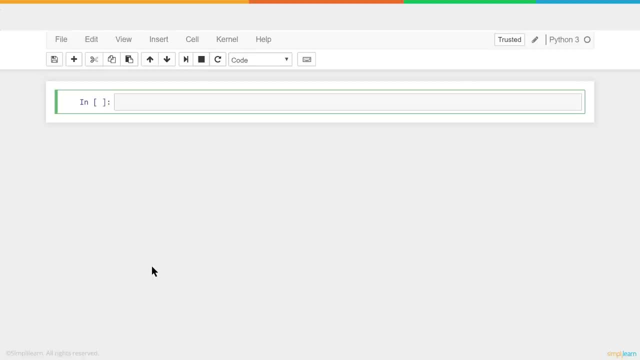 But let's go ahead and switch over there and see what that looks like. So here we are in the Anaconda Python notebook Or Anaconda Jupyter notebook with Python. We're using Python 3.. I believe this is 3.5, but it should work in any of your 3x versions. 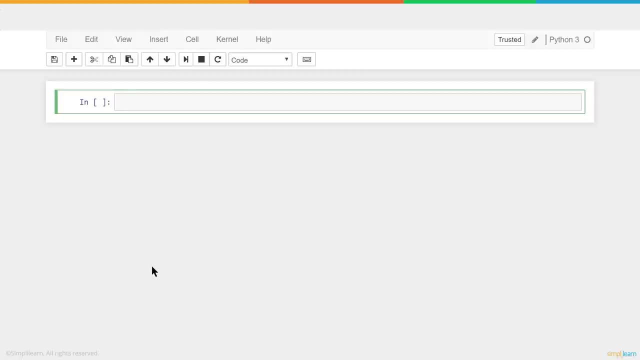 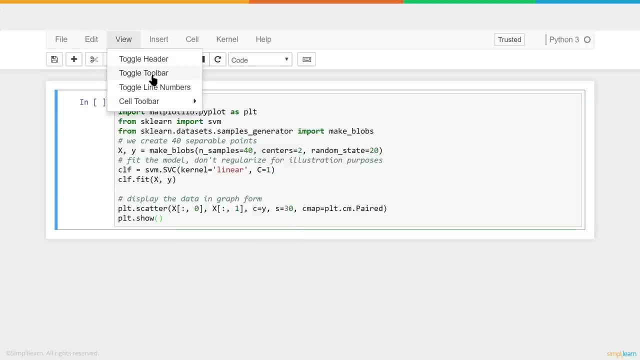 And you'd have to look at the sklearn and make sure if you're using a 2x version or an earlier version. Let's go ahead and put our code in there, And one of the things I like about the Jupyter notebook is I can go up to View. 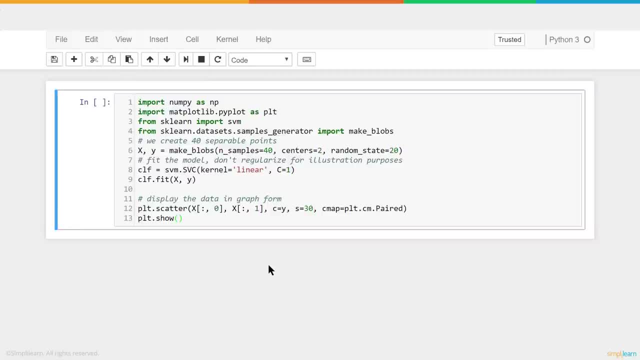 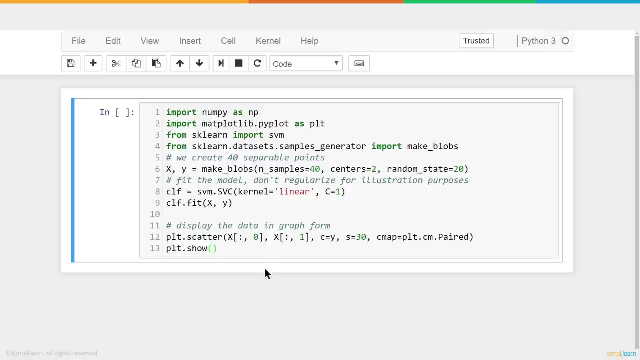 And I'm going to go ahead and toggle the line numbers on to make it a little bit easier to talk about, And we can even increase the size, because this is edited in. In this case, I'm using Google Chrome Explorer And that's how it opens up. 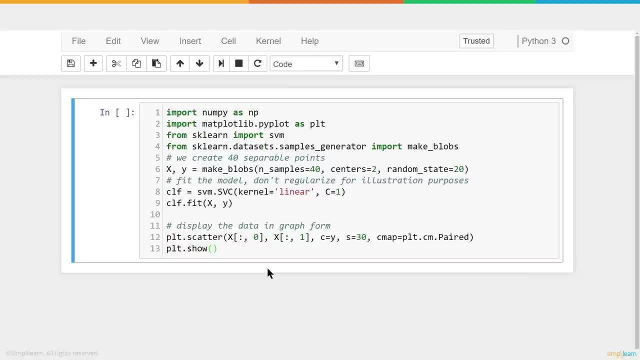 So I'm going to go ahead and do that, And I'm going to go ahead and do that for the editor, although anyone, like I said, any editor will work. Now the first step is going to be our imports, And we're going to import four different parts. 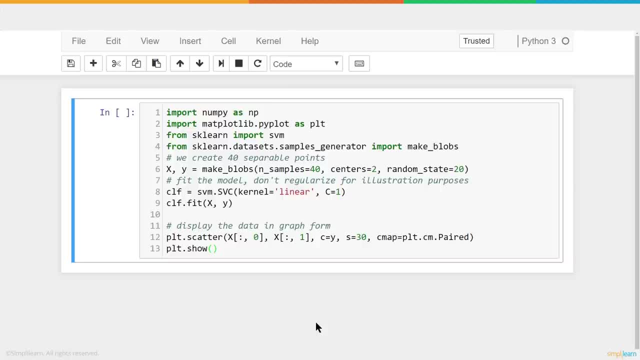 The first two I want you to look at are line 1 and line 2 are numpy as np and matplotlibrarypyplot as plt. Now, these are very standardized imports when you're doing work. The first one is the numbers Python. We need that because part of the platform we're using uses that for the numpy array. 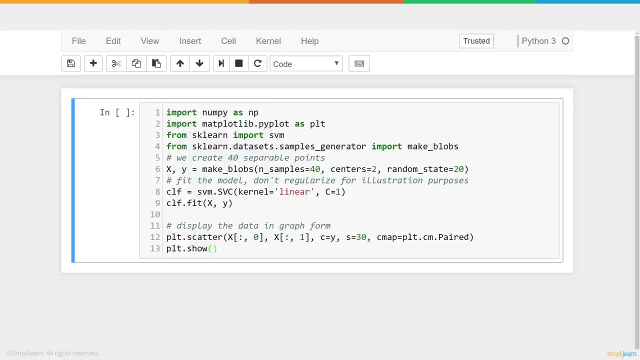 And I'll talk about that in a minute. So you can understand why we want to use a numpy array versus the standard Python array. And normally it's pretty standard setup to use np for numpy. The matplotlibrary is how we're going to view our data. 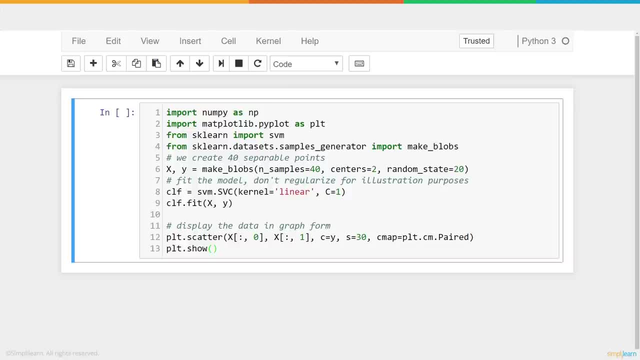 So this has. you do need the np for the sklearn module, But the matplotlibrary is purely for our use for visualization, And so you really don't need that for the SVM. But we're going to put it there so you have a nice visual aid and we can show you what it looks like. 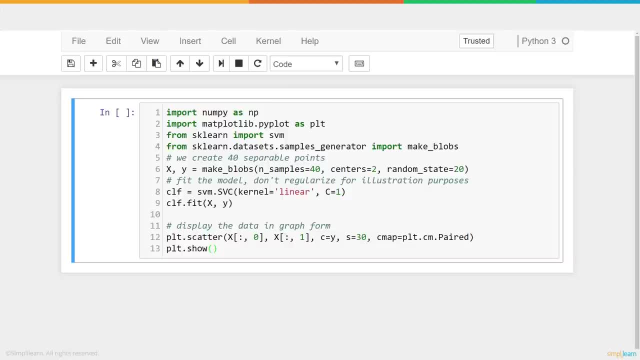 That's really important at the end, when you finish everything, so you have a nice display for everybody to look at. And then, finally, we're going to- I'm going to jump one ahead- to line number four, That's the sklearndatasetssamplesgenerator import makeblobs. 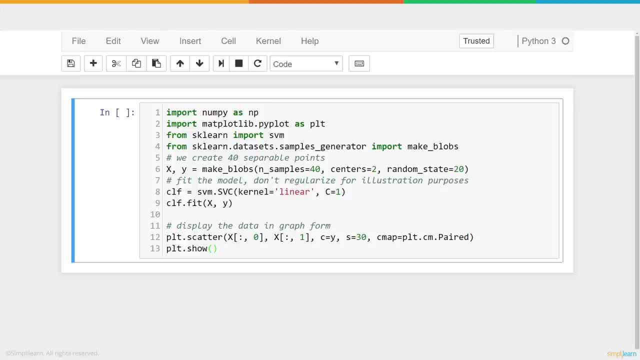 And I told you that we were going to make up data And this is a tool that's in the sklearn to make up data. I personally don't want to go to the zoo, get in trouble for jumping over the fence and probably get eaten by the crocodiles or alligators as I work on measuring their snouts and width and length. 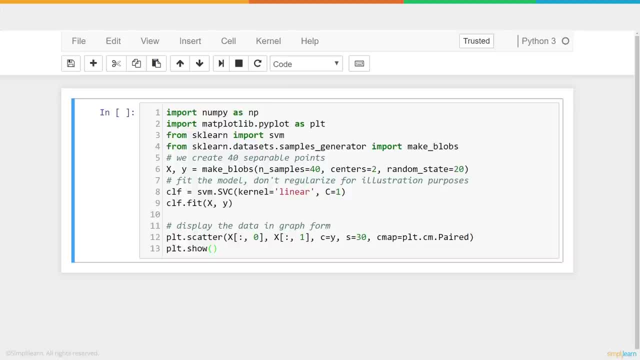 Instead, we're just going to make up some data, And that's what that makeblobs is. It's a wonderful tool. if you're ready to test your setup and you're not sure about what data you're going to put in there, You can create this blob and it makes it real easy to use. 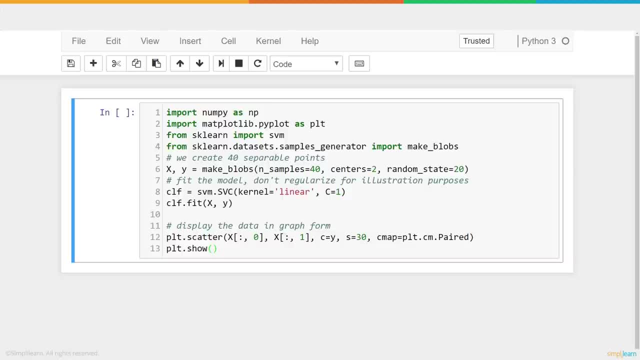 And finally, we have our actual SVM, the sklearn import SVM on line three. So that covers all our imports. We're going to create- remember I used the makeblobs to create data- And we're going to create- a capital X and a lowercase y equals makeblobs. in samples- equals 40.. 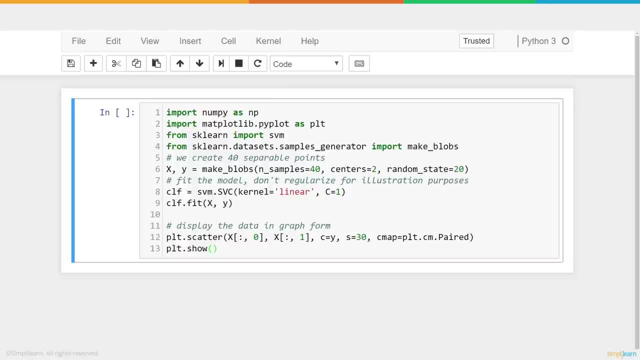 So we're going to make 40 lines of data. It's going to have two centers, with a random state equals two, So each group is going to have 20 different pieces of data in it And the way that looks is that we'll have under X, an XY plane. 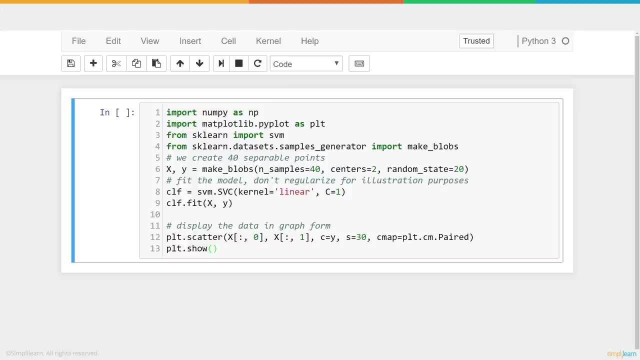 So we'll have two numbers under: X, and Y will be 0 or 1.. That's the two different centers. So we have a yes or no, in this case alligator or crocodile. That's what that represents. And then I told you that the actual sklearn, or the SVM, is in two lines of code. 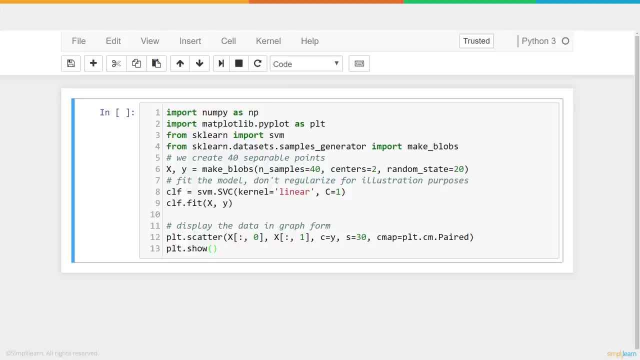 And we see it right here, with clf equals svm, dot, svc, kernel equals linear And I set c equal to 1.. Although in this example, since we are not regularizing the data, since we want it to be very clear and easy to see, 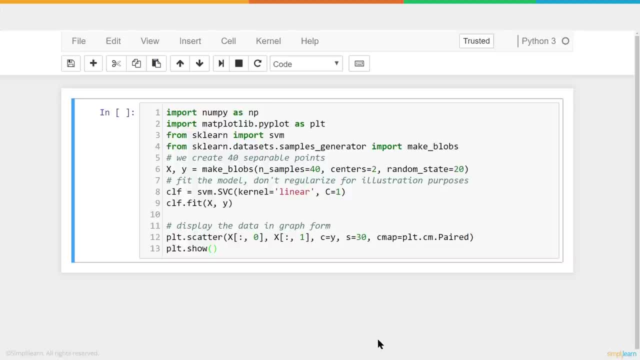 I went ahead. you can set it to 1000 a lot of times when you're not doing that. But for this thing- linear, because it's a very simple linear example- we only have the two dimensions and it'll be a nice linear hyperplane. 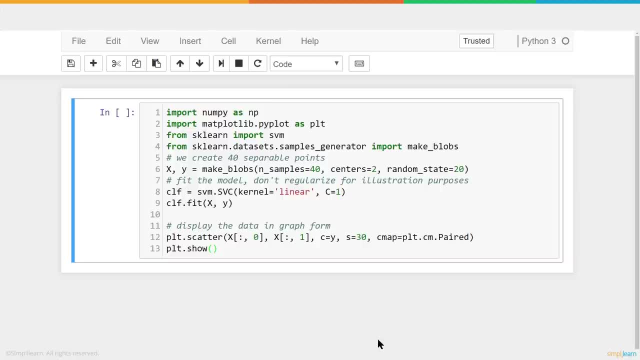 It'll be a nice linear line instead of a full plane, So we're not dealing with a huge amount of data, And then all we have to do is do clf dot fit X, comma Y, And that's it. Clf has been created. 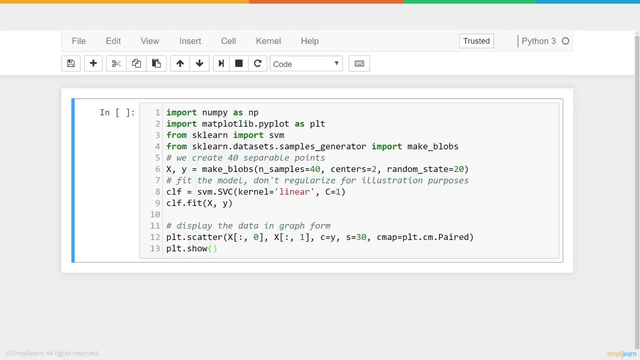 And then we're going to go ahead and display it, And I'm going to talk about this display here in just a second. But let me go ahead and run this code. And this is what we've done is we've created two blobs. 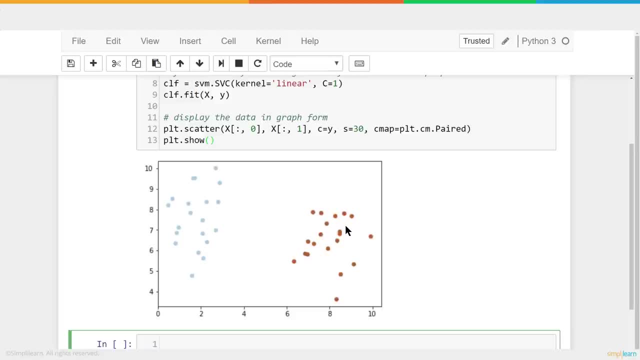 You'll see the blue on the side and then kind of an orangeish on the other side. That's our two sets of data. They represent- one represents crocodiles and one represents alligators- And then we have our measurements. In this case we have like the width and length of the snout. 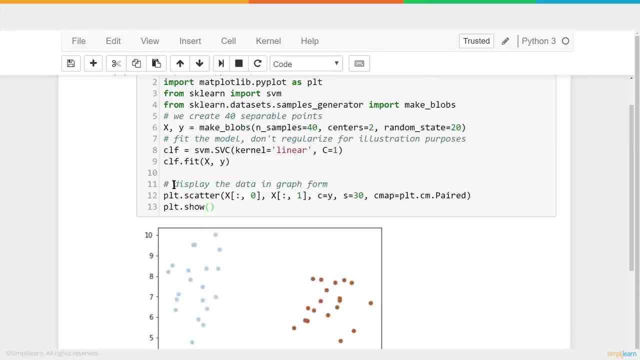 And I did say I was going to come up here and talk just a little bit about our plot. And you'll see, plt, That's our plot, That's what we imported. We're going to do a scatter plot. That means we're just putting dots on there. 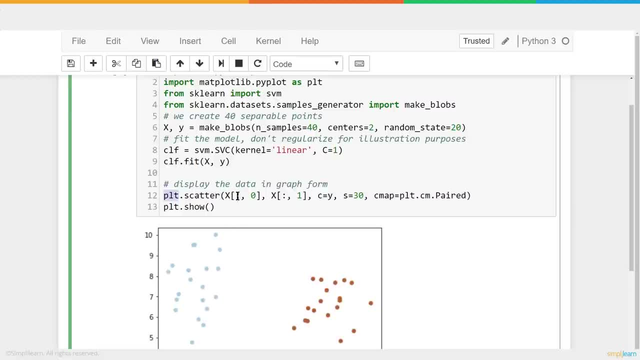 And then look at this notation: I have the capital X and then in brackets I have a colon, comma, zero. That's from numpy. If you did that in a regular array you'll get an error in a Python array. You have to have that in a numpy array. 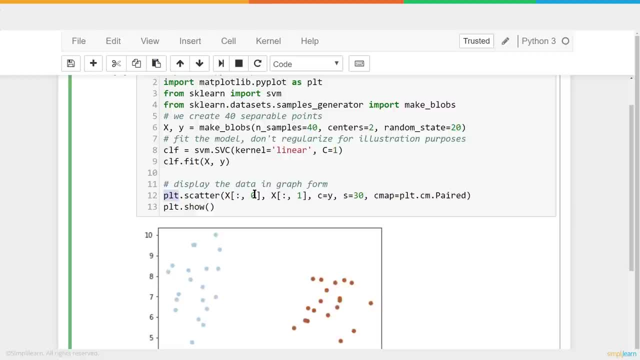 It turns out that our make blobs returns a numpy array, And this notation is great because what it means is the first part is the colon. It means we're going to do all the rows. That's all the data in our blob we created under capital X. 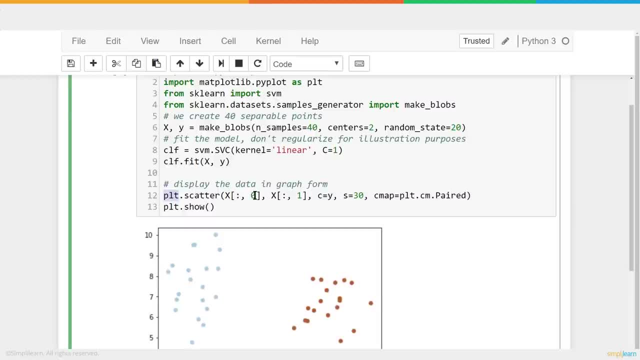 Okay, And then the second part has a comma: zero. We're only going to take the first value And then, if you notice, we do the same thing but we're going to take the second value. Remember, we always start with zero and then one. 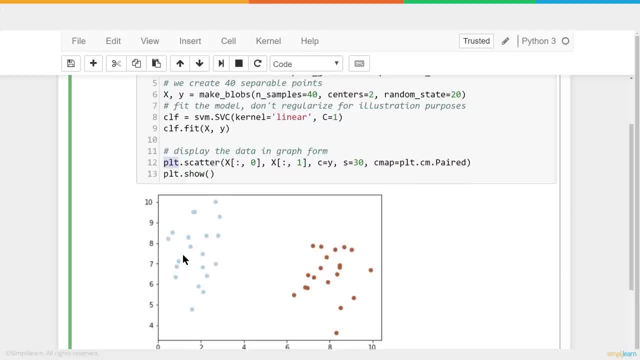 So we have column zero and column one And you can look at this as our xy plots. The first one is the x plot and the second one is the y plot. So the first one is on the bottom. zero, two, four, six, eight and ten. 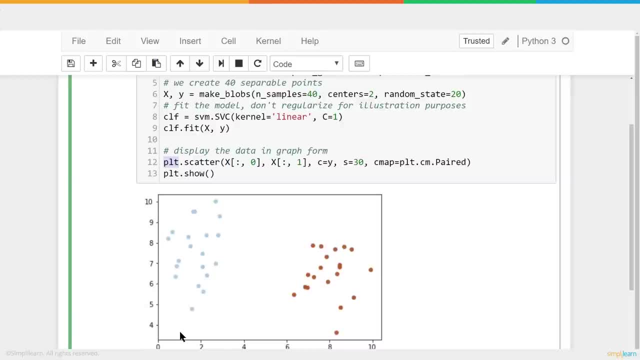 And then the second one, x of the one is the four, five, six, seven, eight, nine, ten. going up the left-hand side, S equals 30, is just the size of the dot, so we can see them. 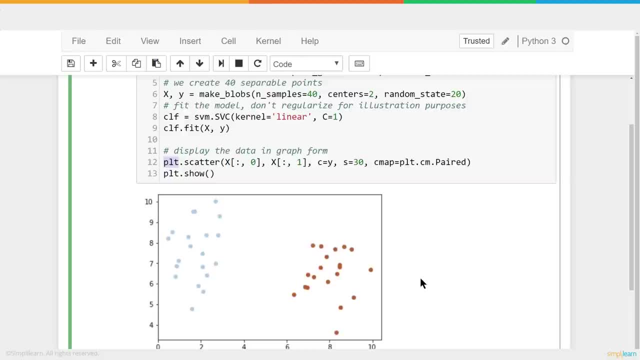 It says real tiny dots, And then cmap equals pltcmpaired, And you'll also see the c equals y. That's the color We're using. two colors, zero one, and that's why we get the nice blue and the two different colors for the alligator and the crocodile. 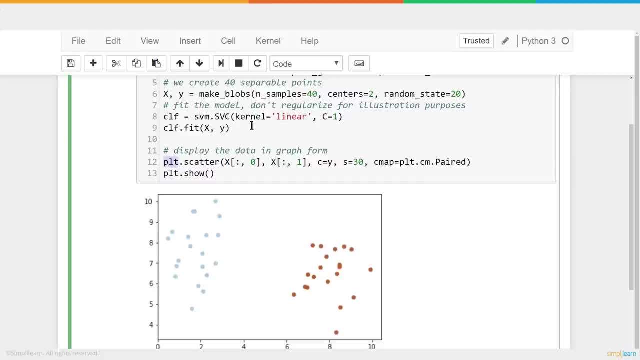 Now you can see here that we did this. the actual fit was done in two lines of code. A lot of times there will be a third line where we regularize the data. We say okay, We set it between like minus one and one and we reshape it. 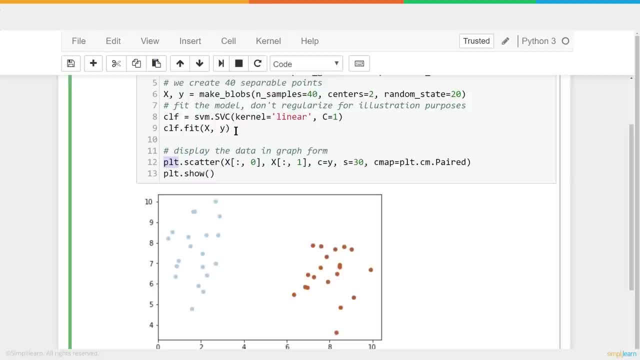 But for this it's not necessary and it's also kind of nice because you can actually see what's going on. And then, if we wanted to, we wanted to actually run a prediction. let's take a look and see what that looks like. 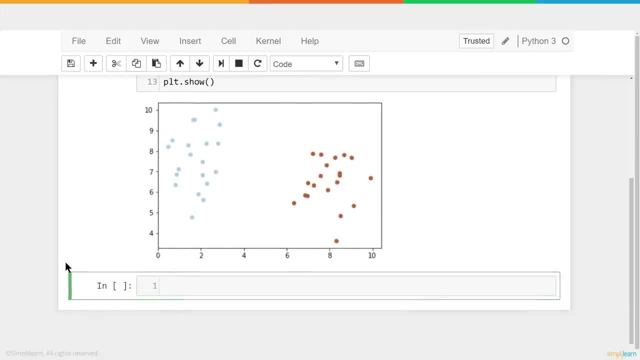 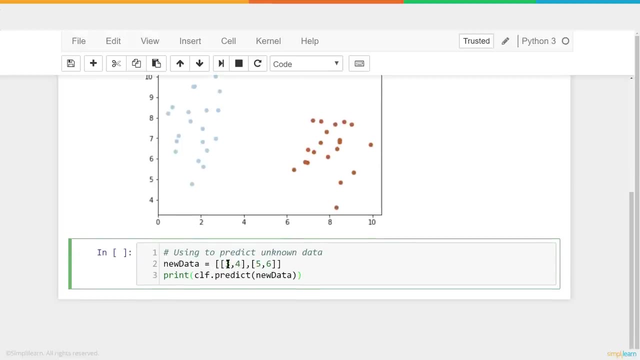 And to predict some new data, and we'll show this again as we get towards the end of digging in deep. you can simply assign your new data. In this case, I am giving it a width and length three, four and a width and length five, six. 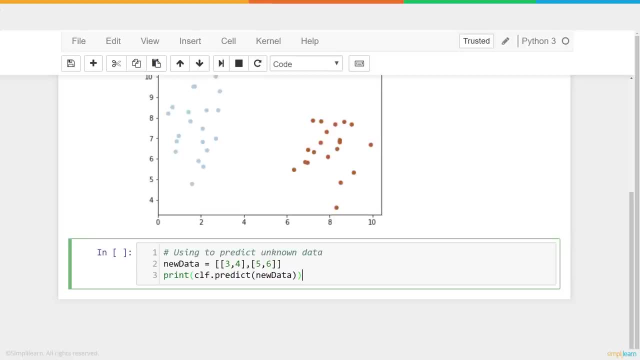 And note that I put the data as a set of brackets and then I have the brackets inside, And the reason I do that is because when we're looking at data, it's designed to process a large amount of data coming in. We don't want to just process one line at a time. 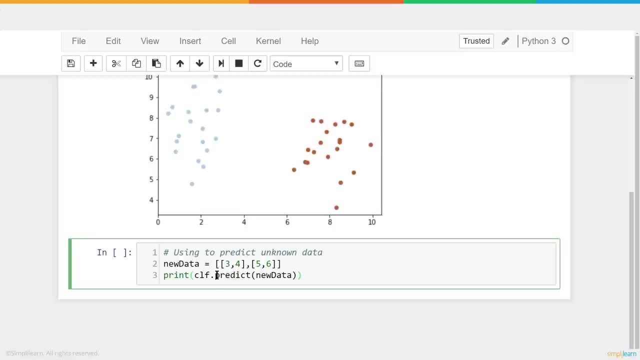 And so in this case I'm processing two lines and then I'm just going to print and you'll see clfpredict new data. So the clf and the predict part is going to give us an answer, And let's see what that looks like. 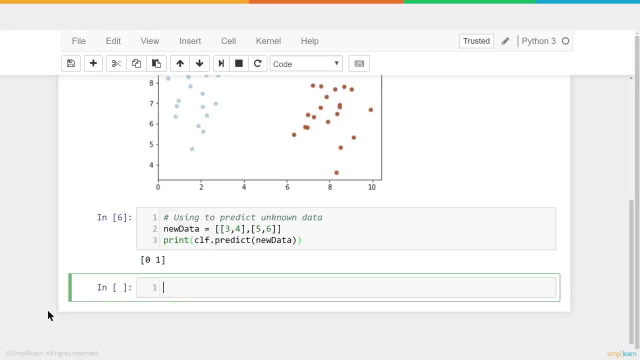 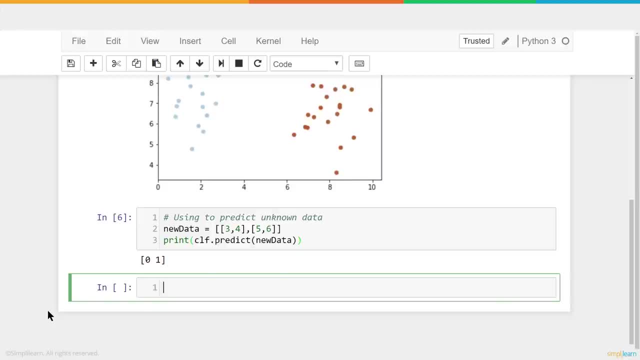 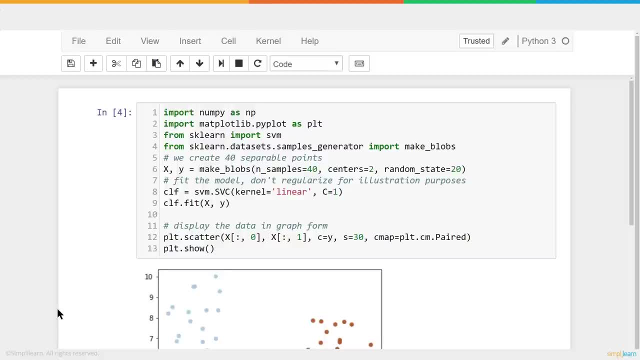 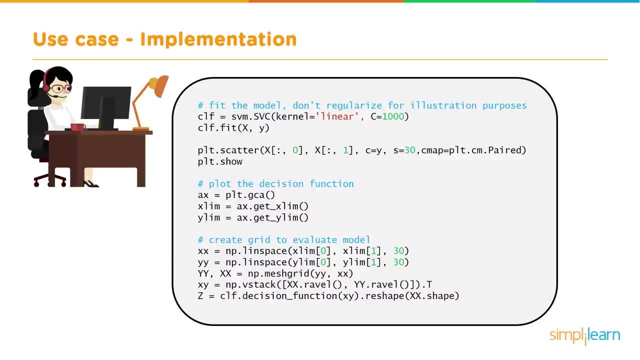 But really we want to dig in and see what is going on behind the scenes And let's see what that looks like. So the next step is to dig in deep and find out what's going on behind the scenes And also put that in a nice, pretty graph. 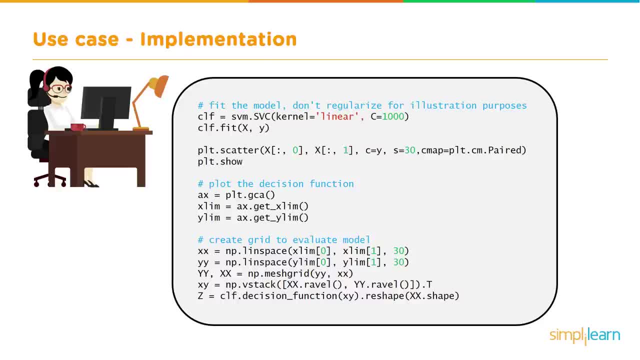 We're going to spend more work on this than we did actually generating the original model, And you'll see here that we go through a few steps And I'll move this over to our editor in just a second. We come in, we create our original data. 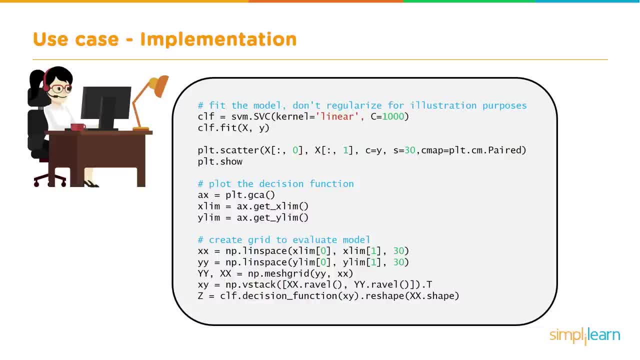 It's exactly identical to the first part And I'll explain why we redid that and show you how not to redo that. And then we're going to go in there and add in those lines. We're going to see what those lines look like and how to set those up. 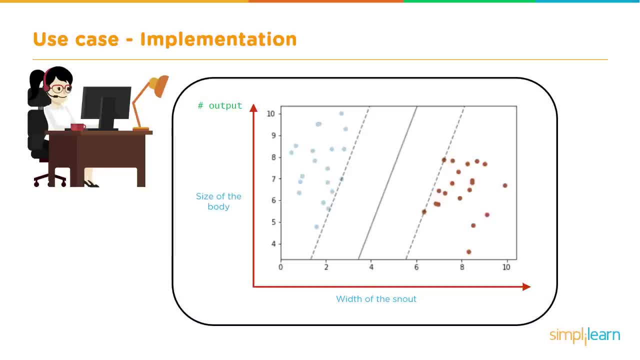 And finally, we're going to plot all that on here and show it And you'll get a nice graph with what we saw earlier when we were going through the theory behind this, where it shows the support vectors and the hyperplane And those are done, where you can see the support vectors as the dashed lines. 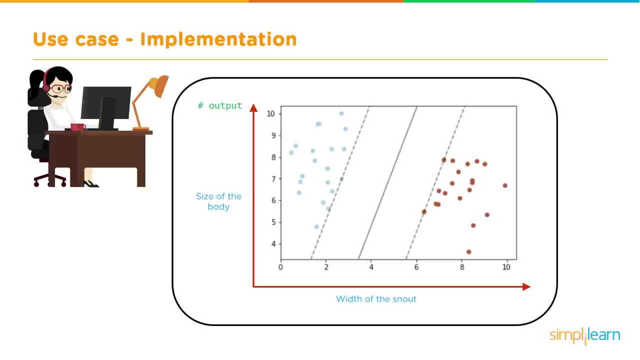 And those are done where you can see the support vectors as the dashed lines and the solid line, which is the hyperplane. Let's get that into our Jupyter notebook. Before I scroll down to a new line, I want you to notice line 13.. 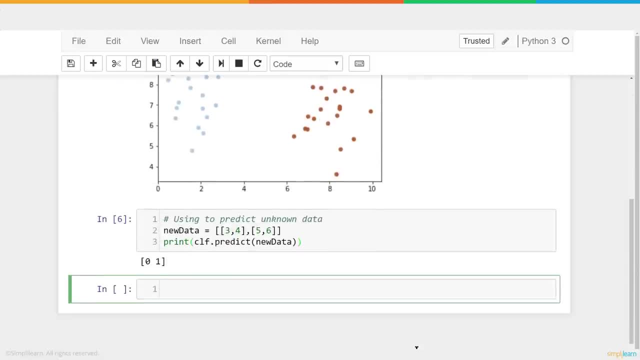 It has plot show And we're going to talk about that here in just a second. But let's scroll down to a new line down here And I'm going to paste that code in And you'll see that the plot show has moved down below. 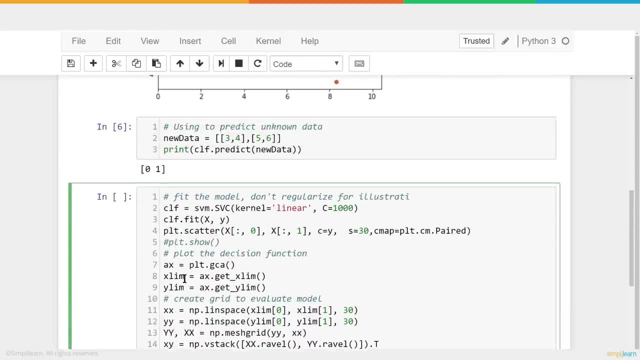 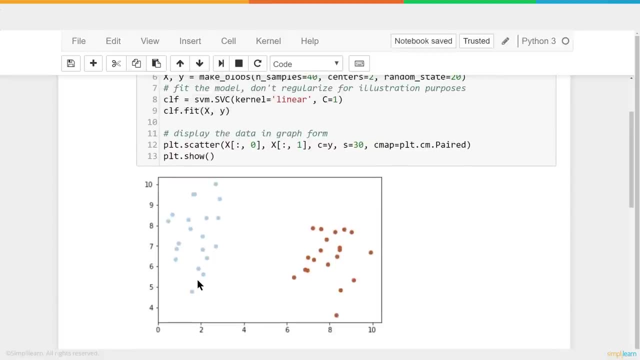 Let's scroll up a little bit And if you look at the top here of our new section, 1,, 2,, 3, and 4 is the same code we had before, And let's go back up here And take a look at that. 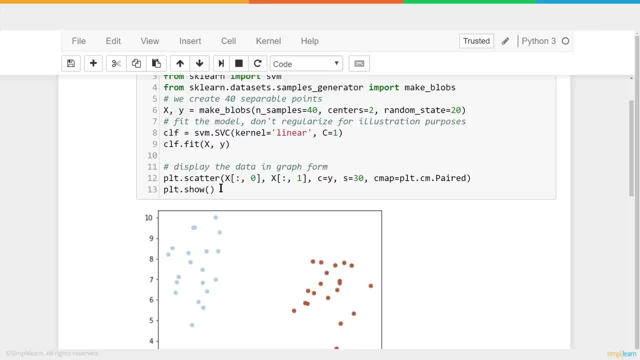 We're going to fit the values on our SVM And then we're going to plot scatter it, And then we're going to do a plot show. So you should be asking: why are we redoing the same code? Well, when you do the plot show, that blanks out what's in the plot. 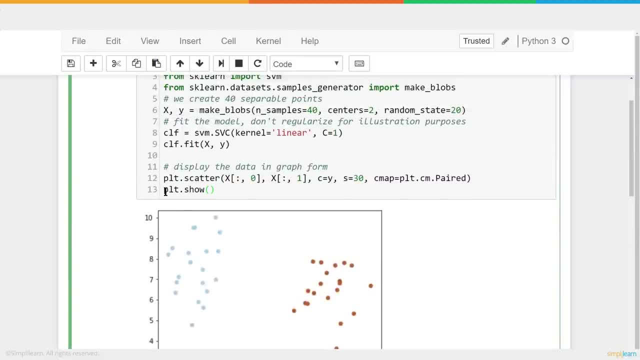 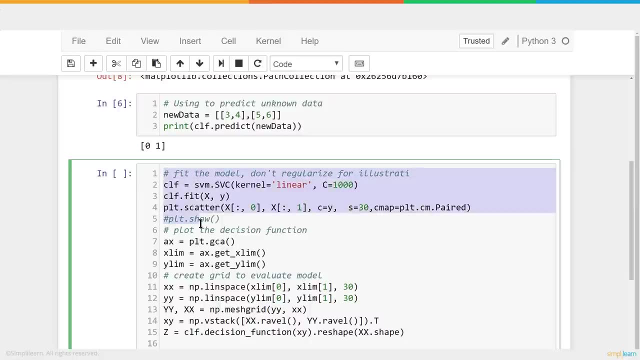 So once I've done this plot show, I have to reload that data. Now we could do this simply by removing it up here, rerunning it and then coming down here, And then we wouldn't have to rerun these first four lines of code. 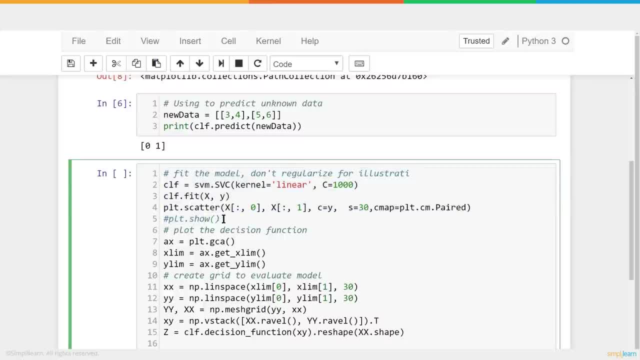 Now in this it doesn't matter too much, And you'll see the plot show. The plot show is down here and then removed right there on line 5.. I'll go ahead and just delete that out of there, because we don't want to blank out our screen. 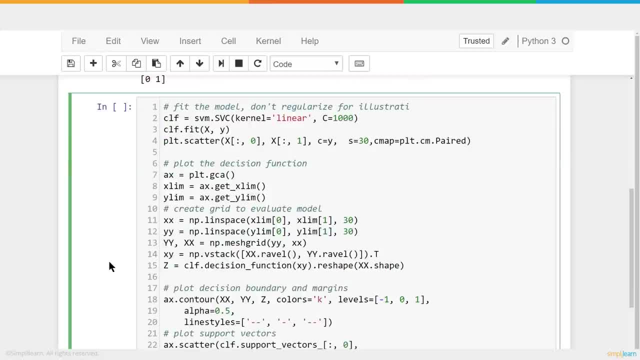 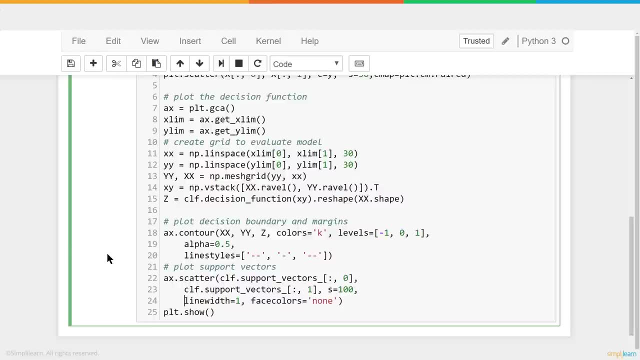 We want to move on to the next setup, So we can go ahead and just skip the first four lines, because we did that before. And let's take a look at the ax equals pltgca. Now, right now we're actually spending a lot of time just graphing. 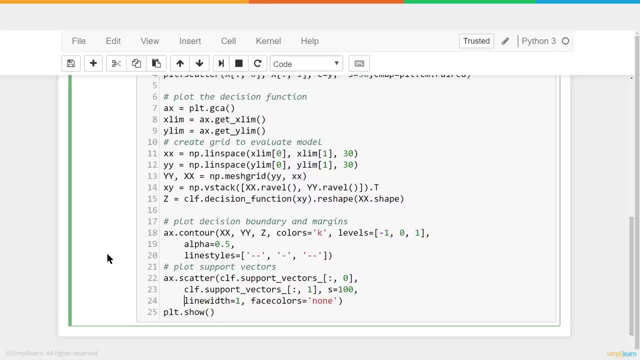 That's all we're doing here. OK, so this is how we display a nice graph with our results and our data. Ax is very standard. No, We use variable when you're talking about plt And it's just setting it to that axis, the last axis in the plt. 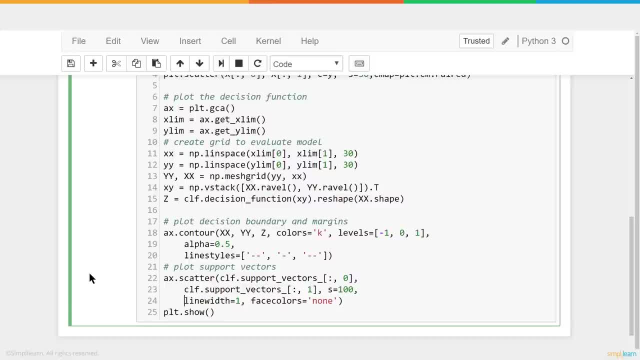 It can get very confusing if you're working with many different layers of data on the same graph, And this makes it very easy to reference the ax. So this reference is looking at the plt that we created, and we already mapped out our two blobs on. 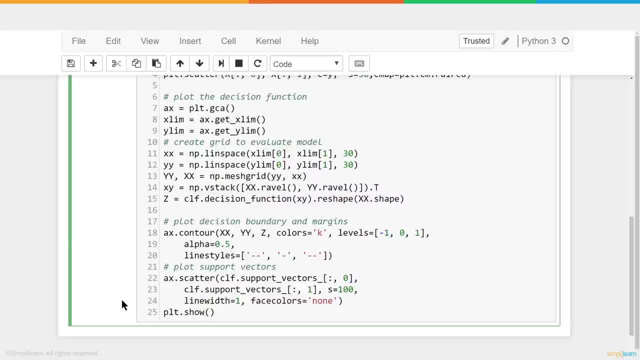 And then we want to know the limits, So we want to know how big the graph is. We can find out the x limit and the y limit simply with the get x limit and get y limit commands, which is part of our matplot library. 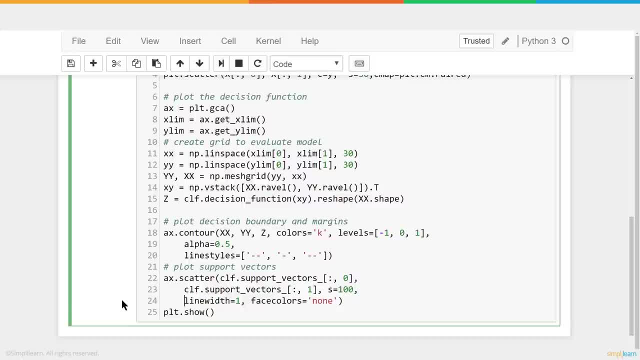 And then we're going to create a grid And you'll see, down here we have. we've set the variable xx equal to nplinespace, x, limit 0,, x limit 1, comma 30.. And we've done the same thing for the y space. 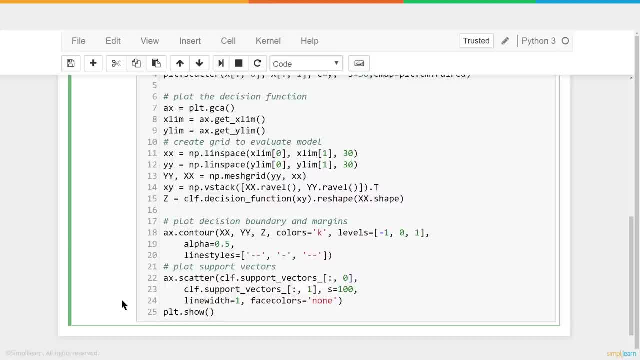 And then we're going to go in here and we create a mesh grid And this is a numpy command. So we're back to our numbers, Python. Let's go through what these numpy commands mean. with the line space and the mesh grid, We've taken xx. 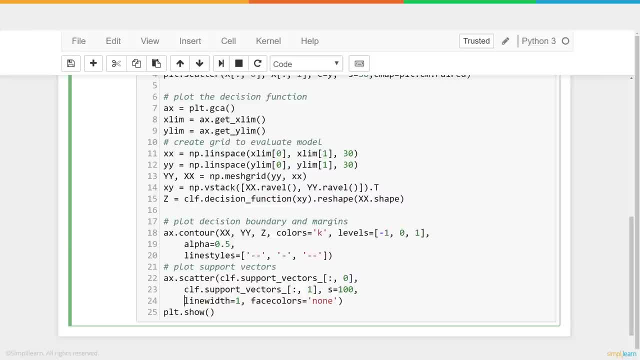 Small s xx equals nplinespace, And we have our x limit 0 and our x limit 1.. And we're going to create 30 points on it And we're going to do the same thing for the y axis. Now, this has nothing to do with our evaluation. 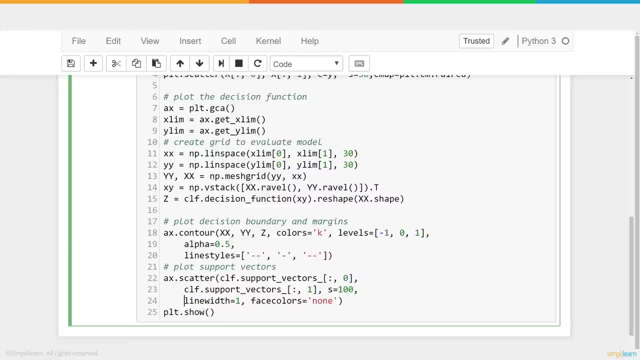 It's. all we're doing is we're creating a grid of data, And so we're creating a set of points between 0 and the x limit. We're creating 30 points And the same thing with the y, And then the mesh grid loops those all together. 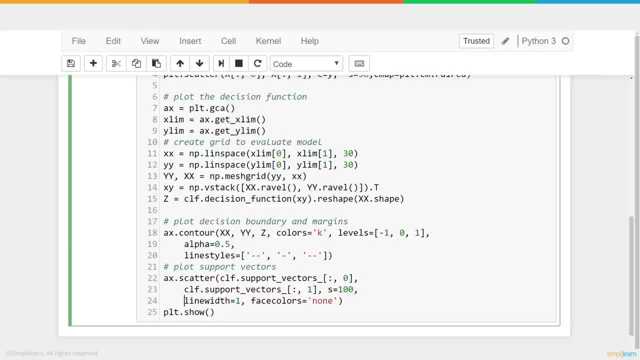 So it forms a nice grid. So if we were going to do this, say between the limit 0 and 10 and do 10 points, we would have a 0, 0, 1, 1, 0, 1, 0,, 2, 0, 3, 0, 4 to 10, and so on. 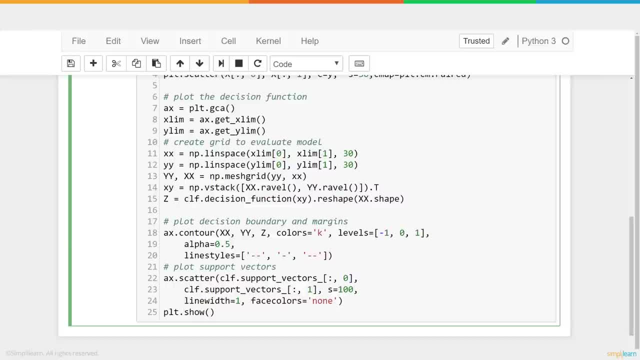 You can just imagine a point at each corner, one of those boxes, And the mesh grid combines them all. So we take the yy and the xx, we created and creates the full grid And we've set that grid into the yy coordinates and the xx coordinates. 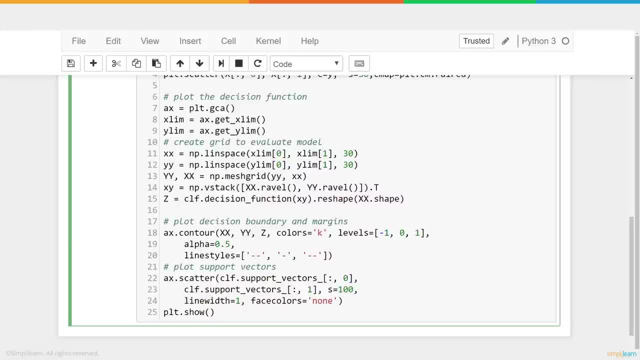 Now remember, we're working with numpy and Python. We like to separate those. We like to have, instead of it being x comma 1, you know, x comma 1.. x comma y, and then x2 comma y2.. And in the next set of data it would be a column of x's and a column of y's. 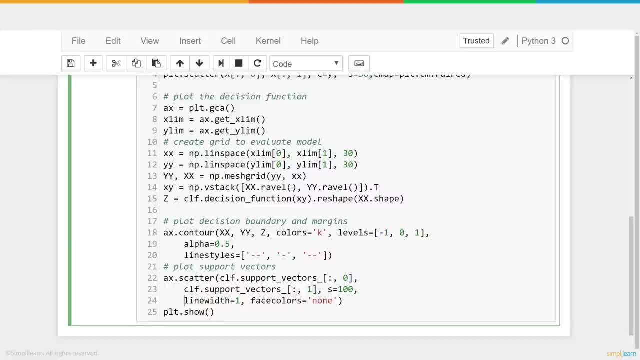 And that's what we have here is, we have a column of y's And we put it as a capital yy, and a column of x's, capital xx, with all those different points being listed, And finally we get down to the numpy v stack. 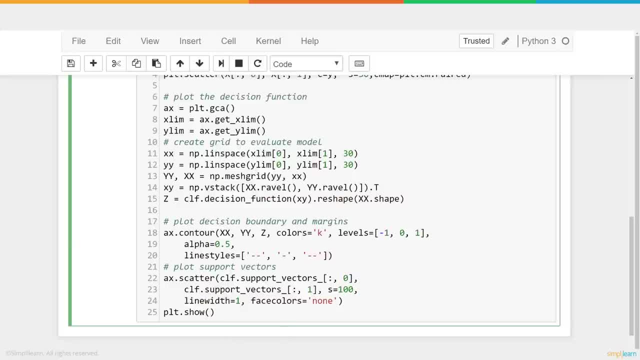 Just as we created those in the mesh grid, we're now going to put them all into one array: xy array. Now that we've created the stack of data points, we're going to do something interesting here. We're going to create a value z. 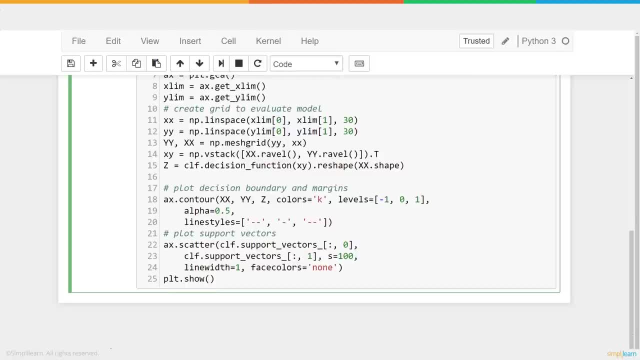 And the z equals the clf. That's our support vector machine. we created and we've already trained And we have a dot decision function And we're going to put the xy in there. So here we have all this data, We're going to put that xy in there, that data, and we're going to reshape it. 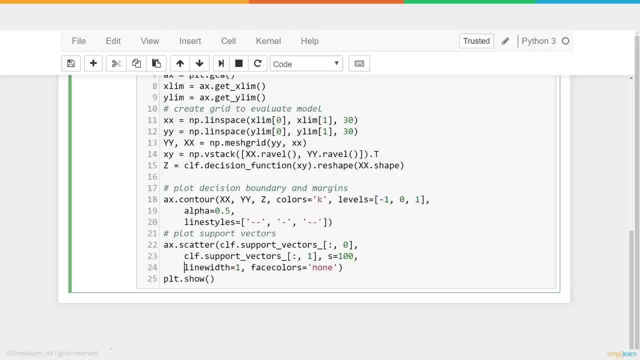 And you'll see that we have the xx dot shape in here. This literally takes the xx, resets it up, connected to the y and the z value. It lets us know whether it is the left-hand side. It's going to generate three different values. the z value does. 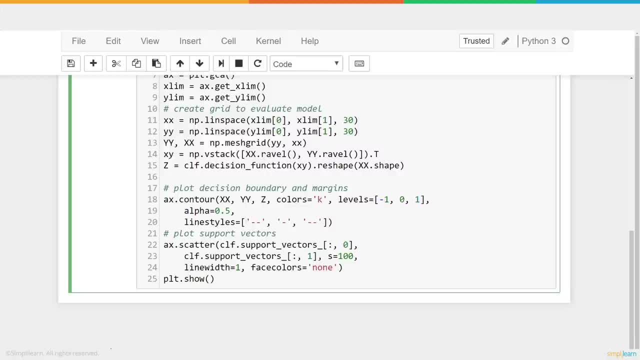 And it'll tell us whether that data is a support vector to the left, the hyperplane in the middle or the support vector to the right. So it generates three different values for each of those points, And those points have been reshaped so that they're right on a line. 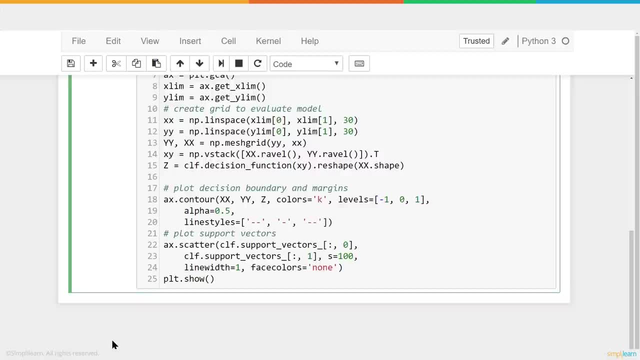 on those three different lines. So we've set all of our data up, We've labeled it to three different areas and we've reshaped it And we've just taken 30 points in each direction. If you do the math, you have 30 times 30, so that's 900 points of data. 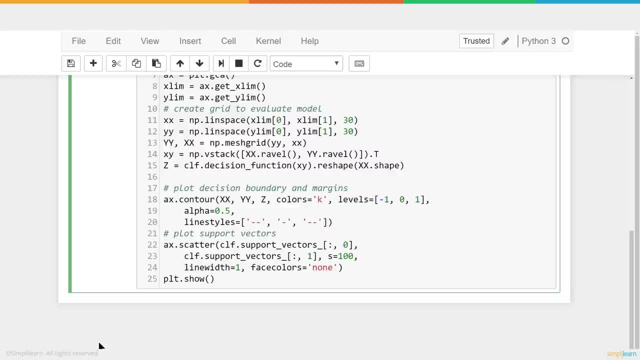 And we separated it between the three lines and reshaped it to fit those three lines. We can then go back to our map plot library. We've created the ax and we're going to create a contour, And you'll see, here we have contour, capital xx, capital yy. 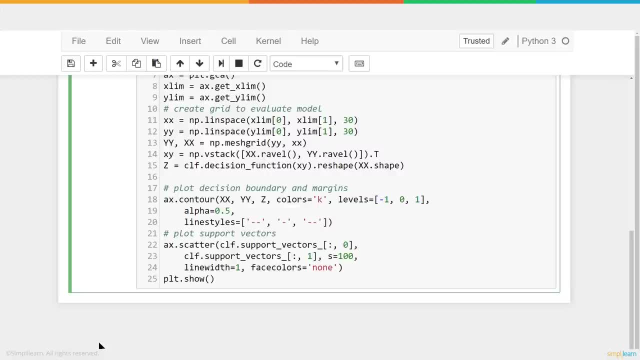 These have been reshaped to fit those lines. Z is the labels. So now we have the three different points with the labels in there And we can set the colors. equals k. And I told you we had three different labels, but we have three levels of data. 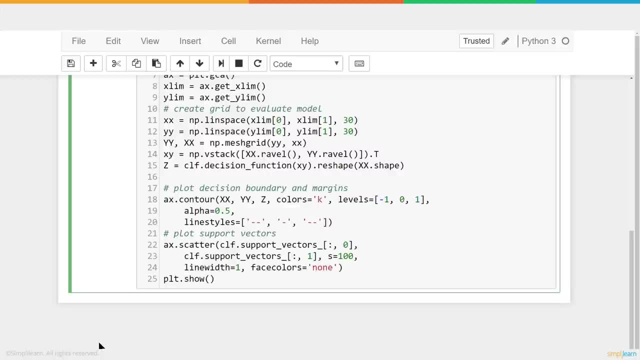 The alpha just makes it kind of see-through. So it's only 0.5 of the value in there. So when we graph it, the data will show up from behind it wherever the lines go. And finally the line styles. 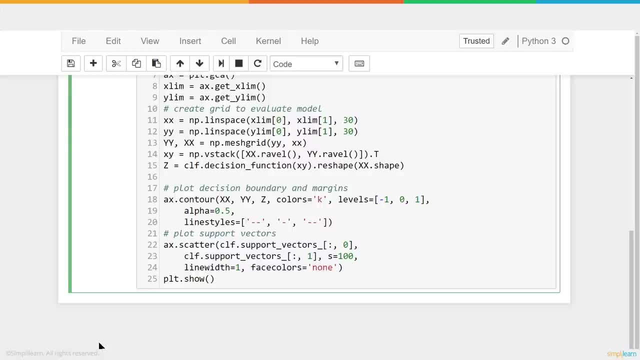 This is where we set the two support vectors to be dash, dash lines, And then a single one is just a straight line. That's what all that setup does. And then, finally, we take our axscatter. We're going to go ahead and plot the support vectors. 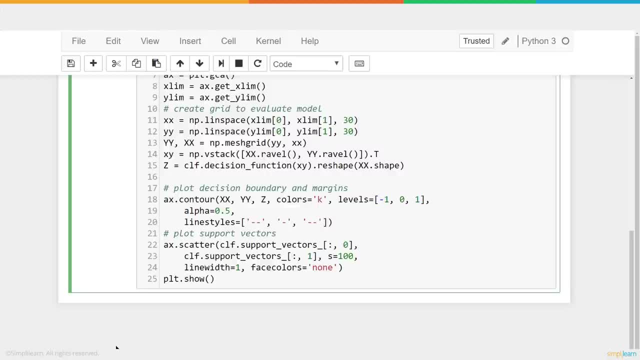 but we've programmed it in there so that they look nice like the dash dash, The dash dash line and the dash line on that grid. And you can see here, when we do the clfsupportVectors, we are looking at column 0 and column 1.. 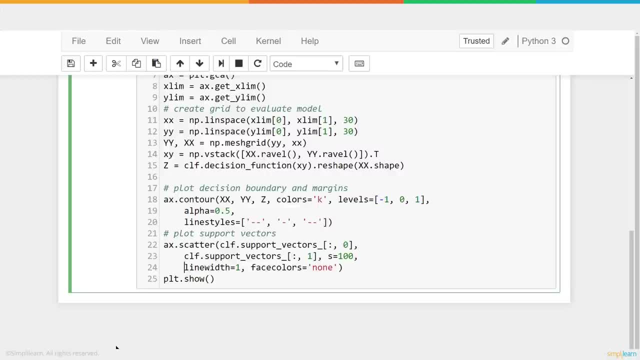 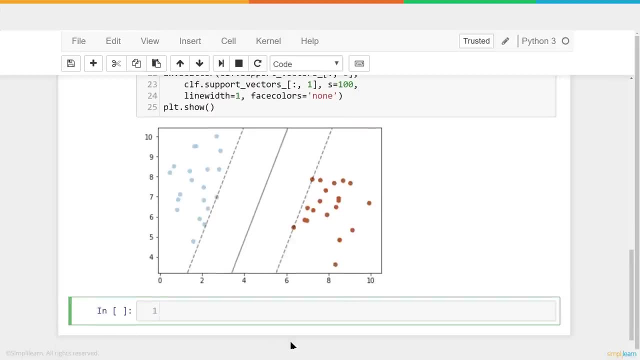 And then again we have the s equals 100.. So we're going to make them larger And the line width equals 1.. Face colors equals none. Let's take a look and see what that looks like when we show it And you can see when we get down to our end result.